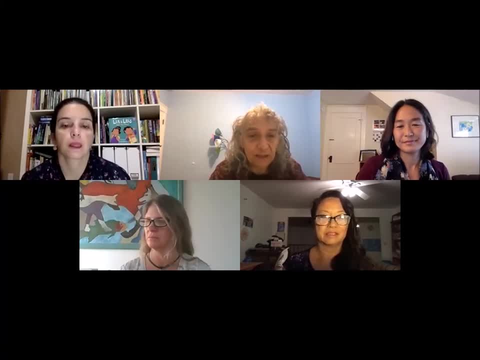 there are some big gaps in what's in print. A lot of the math picture books have animal and white main characters, but there are very few with main characters of color. Most math picture books center on counting or shapes, but there are other math topics that are. 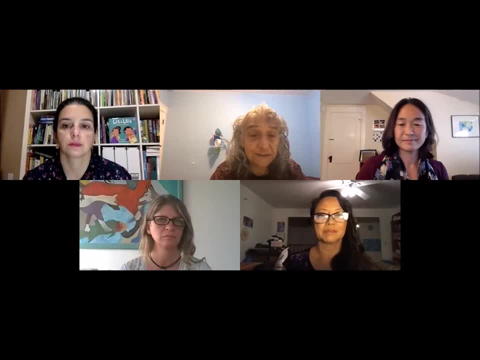 also very important for children's math, So I'm going to give you a little bit of a look at some of the books that are important for young children to experience, And most of the books are more about math than about great stories. Storytelling. math books offer a different vision of what math is. 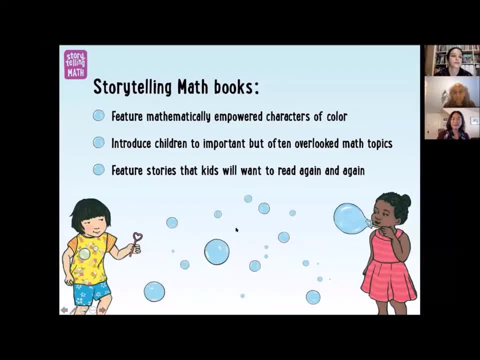 and who is a mathematical thinker? Okay, thanks, Marlene. Storytelling math books star main characters of color and most of the books are written by own voices, authors, so authors writing about their own culture. Storytelling math books feature important but 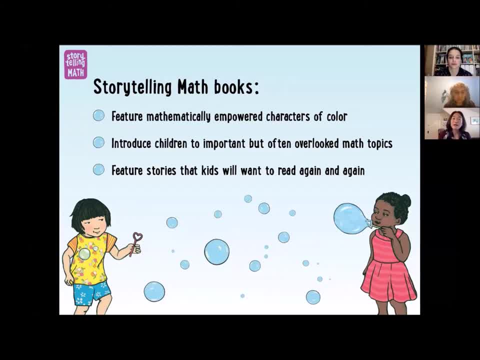 overlooked math topics like patterns or spatial relationships, Topics that research shows are really important for kids in all subjects, including reading. The books also feature stories that kids are going to want to read again and again. You know we expect picture books to be emotionally resonant and compelling and fun. 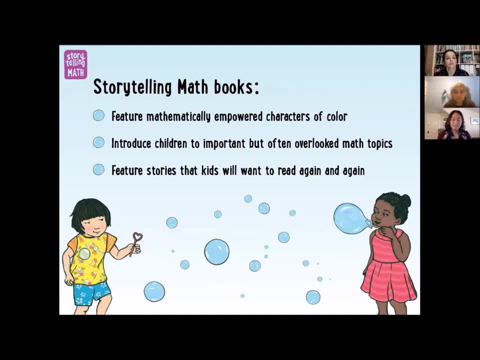 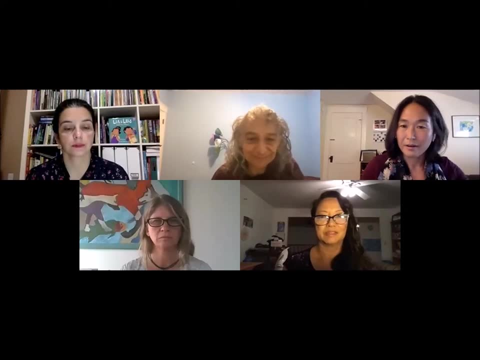 and why not expect the same of math picture books? So the first six storytelling math books are available. now Let me- and they are: oh gosh, okay, sorry, I'm trying to share my screen. okay, can you see my screen? not yet, no, no, okay, all right. so 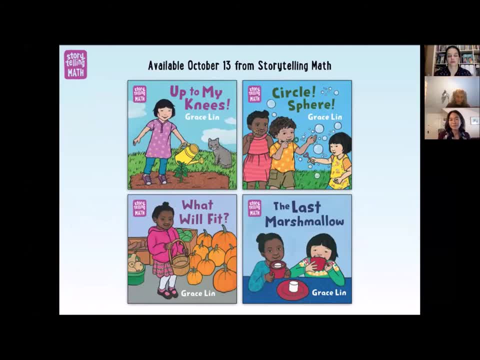 okay, so we have these four really adorable, wonderful board books by Grace Lin Caldecott, Honor winner and real superstar. She explores the seasons in these books and features three characters of color- Olivia, Mae and Manny- and they just explore everyday math through. 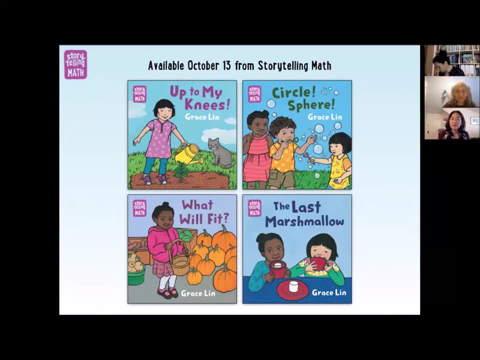 activities that kids do all the time, you know: blowing bubbles, sharing cocoa. it's um, I am, I. You can hear we've got videos on our website of grace talking about the making of the books, and that's she's just. she speaks about diversity in math, really fabulously. 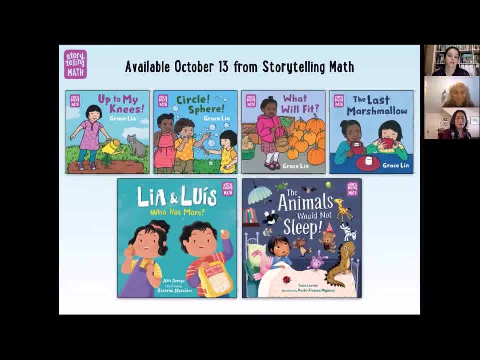 We also have our first two storytelling mass picture books- Very wonderful, funny, touching stories by Anna and Sarah and they'll be talking about those in a little bit. And our third storytelling math picture book by Natasha is Luna's Yum Yum To The Sun and that is coming on December 22nd. 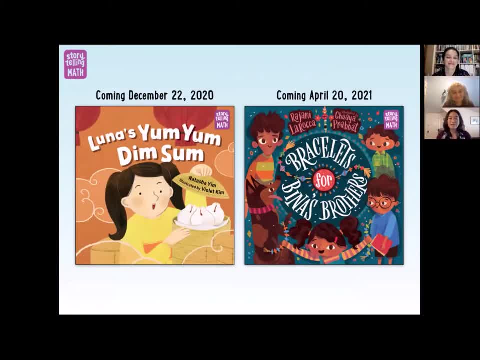 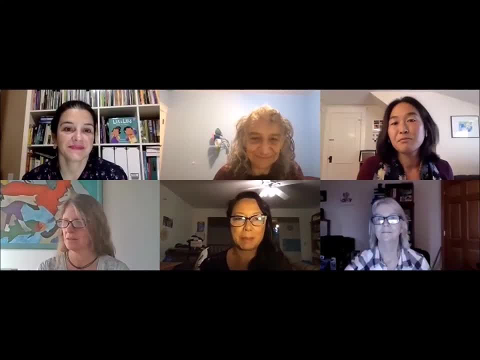 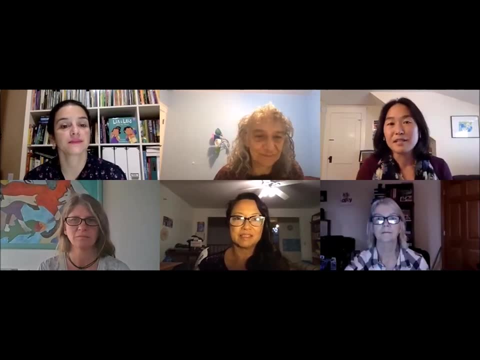 just in time for Chinese New Year, So I'm going to start off. let me stop sharing my screen. I'm going to start off with some questions for Anna, So please feel free to add your own questions in chat and we'll ask them of Anna, because we really want this to be a conversation. 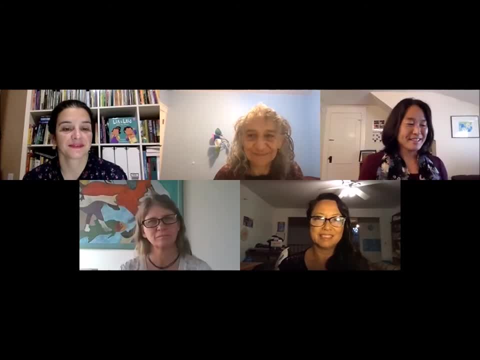 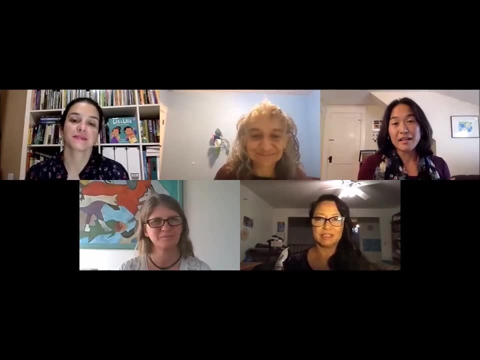 So, oh, you know I should introduce you Anna. So Anna is originally from Brazil and she moved to the United States to pursue a master's of education degree, And here she fell in love with children's books and became a writer. She is the author of several titles, including The Soxies. 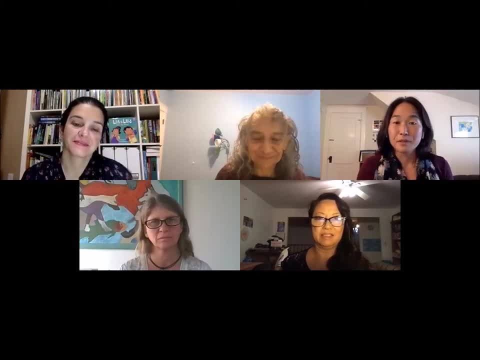 A Soccer Story, a winner of an International Latino Book Award, And now she is the author of the wonderful Leah and Luis. So, Anna, how did you come to write Leah and Luis? Hi, Hi, everyone, Hi, Erin, I see you So. 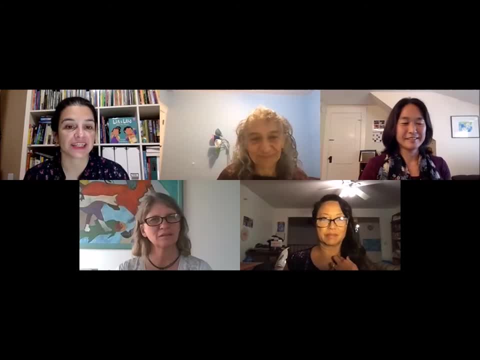 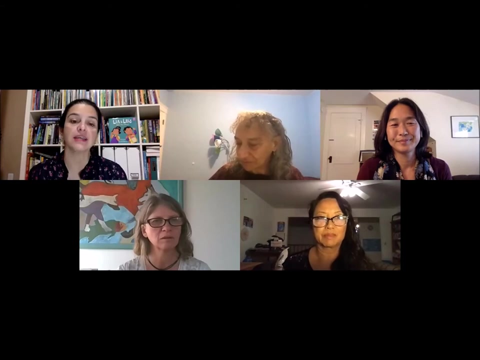 I think I really was at the right place at the right time because we matched- I don't know if you remember, but I think it was PLA in Denver- And while we still could have live events right, which was wonderful- And you mentioned that you guys were putting together the series and that 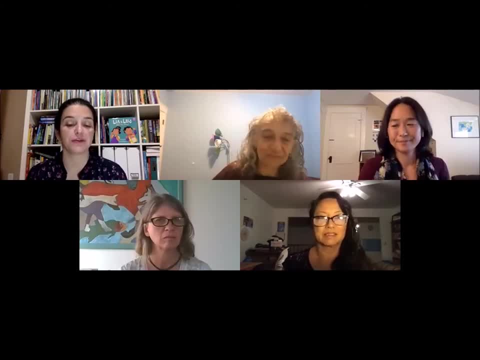 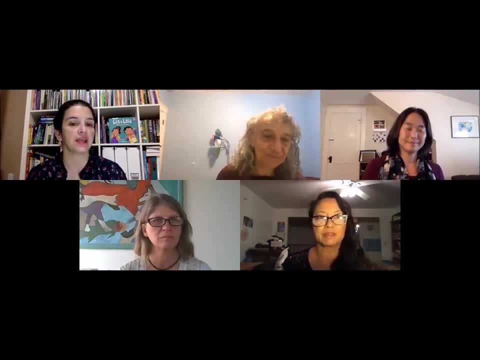 ask you to send me the call for support. So I'm going to ask you to send me the call for support And I really think that if I hadn't met you, maybe I wouldn't have tried, just because I had never written a story based on a prompt before, So that was a little intimidating to me. 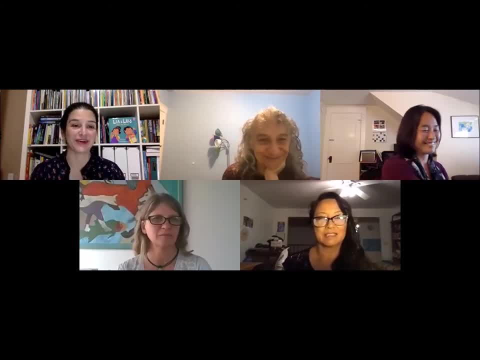 But anyway. but I tried right And I am so happy that I tried. I wrote two stories. I don't know if everybody's familiar with how these series we split together, But from what I understand there were over 500.. 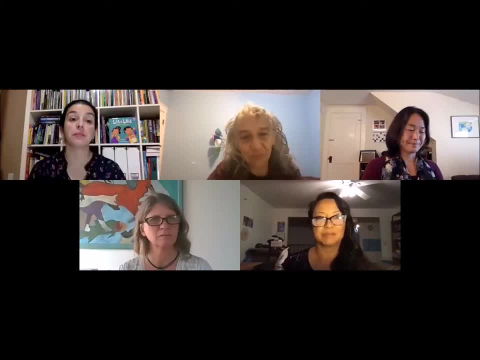 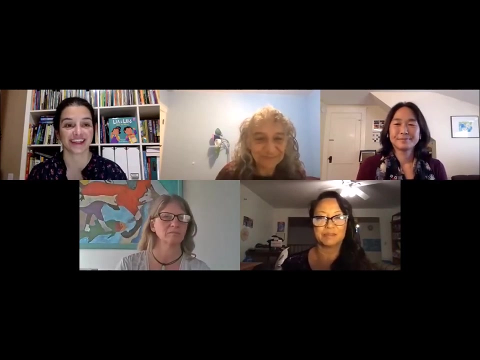 submissions. I submitted two stories and what in the end week was the one picked. so so that's how I got involved and I was really excited about the premise of the, the series, and really excited to know I had been, my manuscript had been chosen. so thank you for the opportunity. well, we were so pleased when we saw your 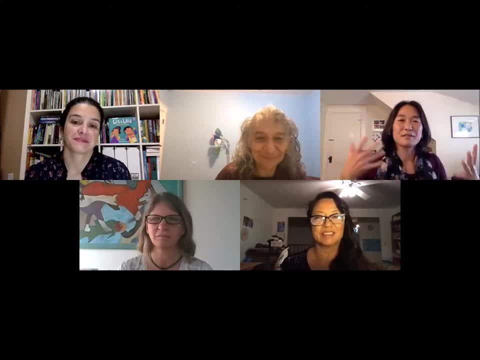 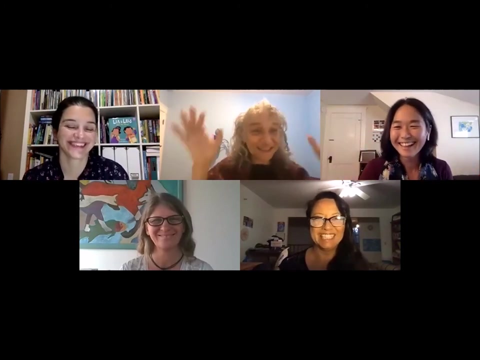 manuscript, Anna. I just it really stood out because you you wrote with such a. you have these characters who came to life on the page and the. the writing is very light and playful and and Marlenia's like she gets the math. this is exactly what we wanted. 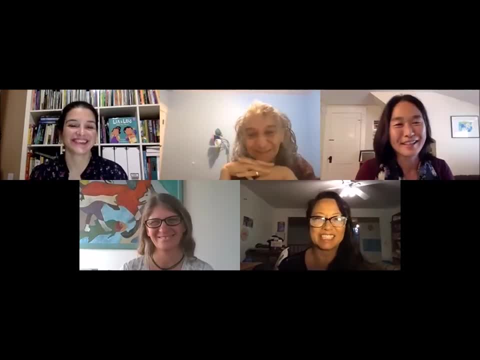 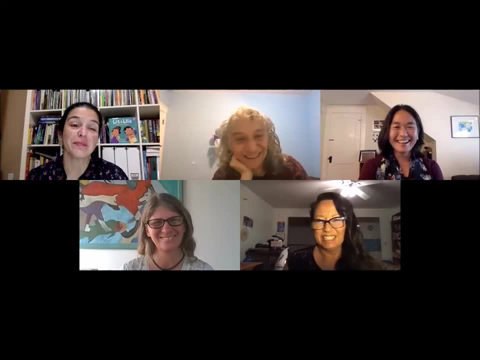 but we are thrilled you found us. I really like Brazilian snacks, yeah, and I am like in a place where i have to drive about over an hour to get any brazilian snacks. so i was riding it and i was so happy that i had to drive there and get me some to make sure that i had all the 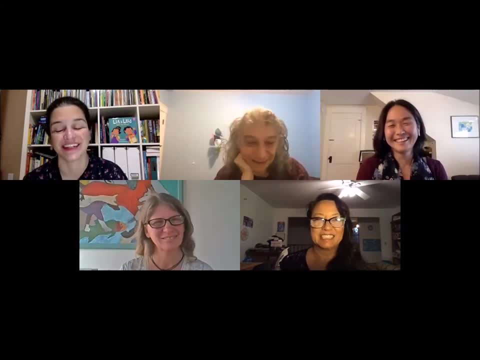 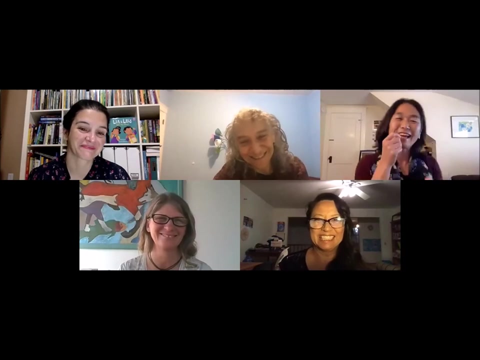 measures, correct, correct and everything and so, yeah, so it was fun to ride and participate in the project, and very yummy too, yeah, and, and anna, you sent some some of the snacks to marlene and me and so we were in the office. you know, measuring and tasting. it was a very fun process. but 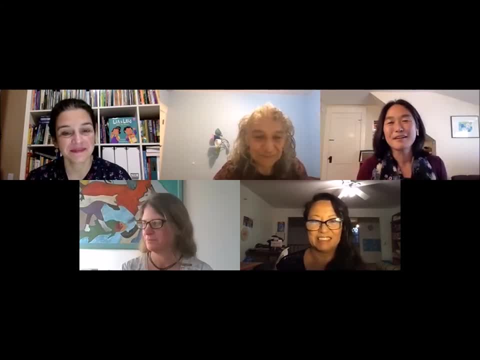 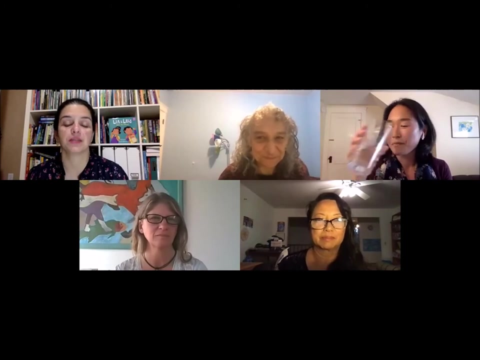 so could you tell us uh more about leon luis, like, what is the story about and what are the? who are the characters? sure, so the main characters are, uh, lee louise, who are brazilian american twins. um, and the plot of the story, the, the, is pretty much they are uh, uh, arguing about who has more. 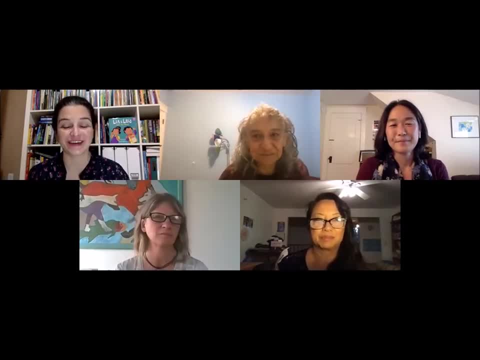 snacks right. so i don't know if you guys did that when you were younger, but i know that i did uh compare how much i, how much food i had in comparison to my uh brothers and uh, just to annoy them, i think i was a little bit, i had a little bit of louise in me, um and so and so anyway, 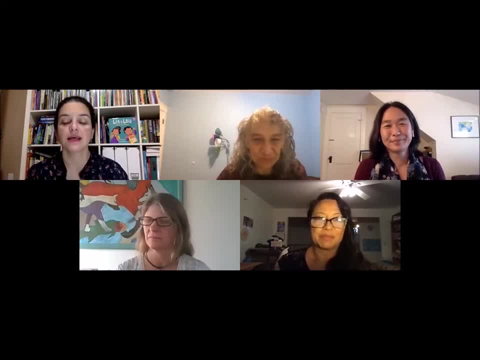 so that's what they're trying to do. they're trying to compare the snacks, uh, and find out who has more. but they are comparing through different methods. they're measuring it in different ways, so they're figuring out which one is the tallest, which one is the deepest. this one looks bigger, uh, uh, but this one has more. 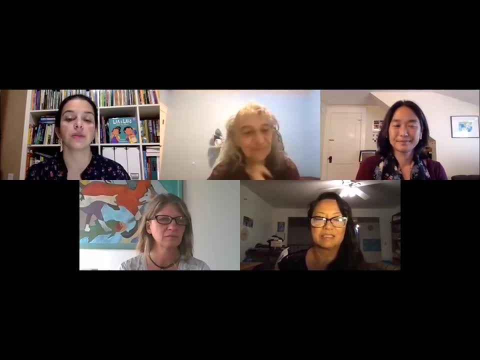 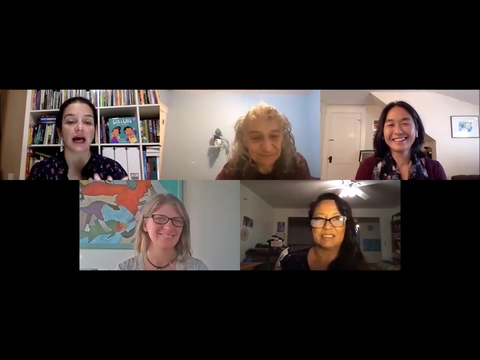 in quantity. so they're figuring out all these different ways to, to, to come up with an answer to their question, and eventually is it okay to uh sort of uh, uh, tell the the ending of the story. i guess it's okay, right? so eventually they decide that uh, oh, we can weigh them and that's how they. 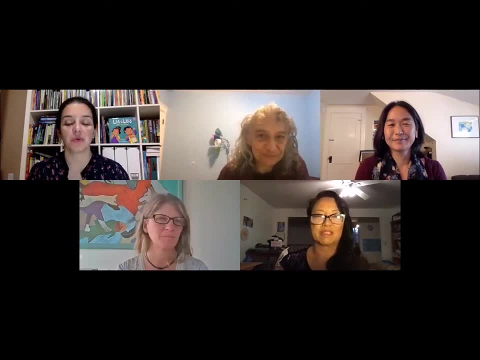 uh, figure out who has more, and so what i think is fun about it is that, uh, really, there are so many ways for you to compare. uh, uh, two things right. i mean, if you're comparing apples to apples, then you can compare it by quantity, but if you're comparing apples to oranges, then you know it might. 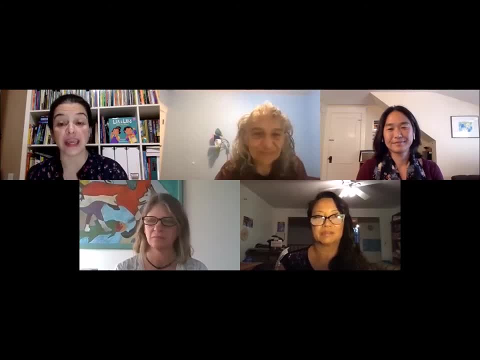 be better to do it via, to figure out the weight or or if you're comparing something else. so it depends really on what you're comparing. um, so that's why i thought it was a a good way to to approach the mathematical uh plot of you know, of the stories. yeah, so that's how you? yeah, could you. 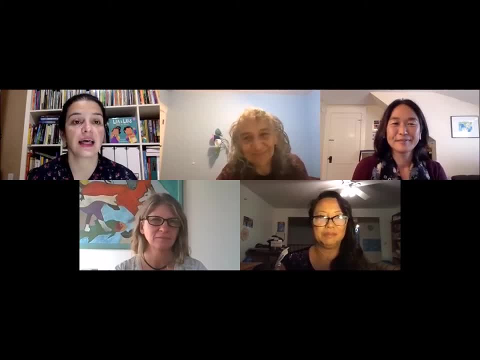 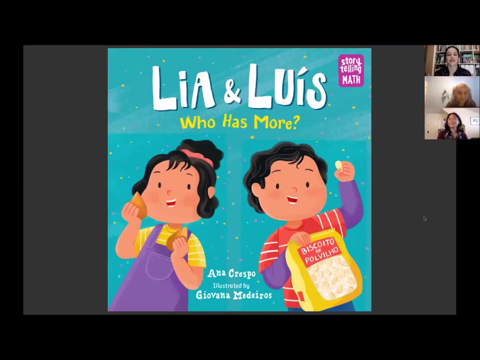 read um, read a few pages maybe. sure, beginning of the book. let me just figure it out here really quick. i, i practiced and, uh, i believe i know how to do it, but, okay, can you see it? yes, okay, so, uh, the book is illustrated by giovanna meteros, who is also um brazilian and um published, of course, by charles. 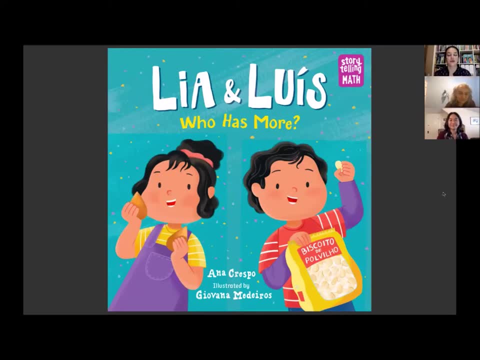 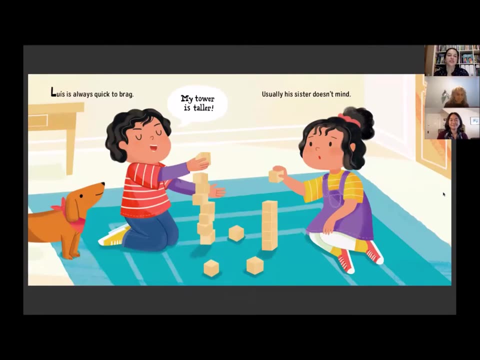 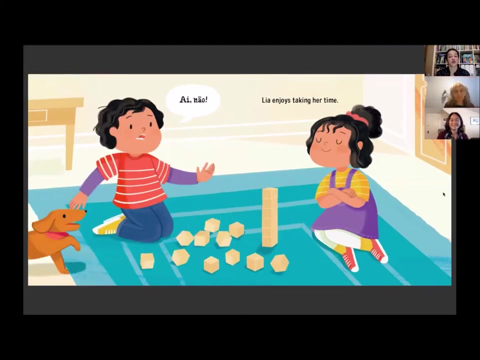 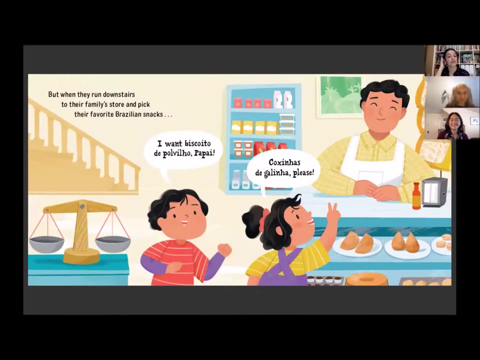 bridge, so let's go ahead and lee and louise- who has more? okay, louise is always quick to brag. my tower is taller. usually his sister doesn't mind. leah enjoys taking her time, but when they run downstairs to their family's store and pick their favorite brazilian snacks, 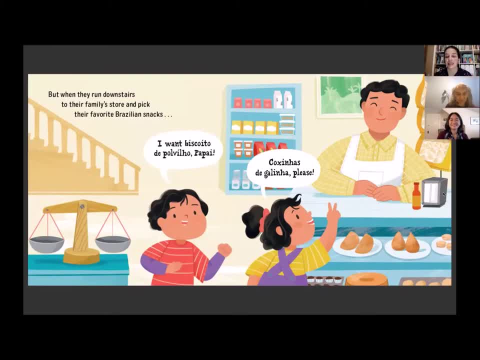 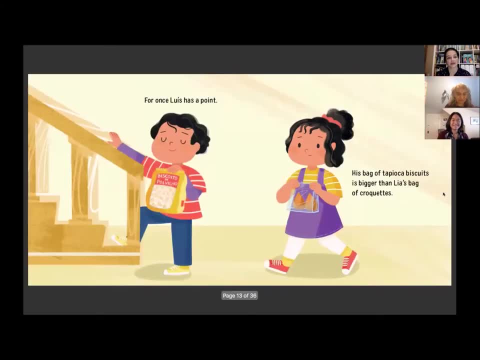 i want biscoito de povilho, papay coxinhas de galinha. please louise starts bragging. i have more and leah doesn't like it. for once, louise has a point. he's bag of tapioca biscuits is bigger than leah's bag of croquettes. it is taller, wider, deeper, louise. 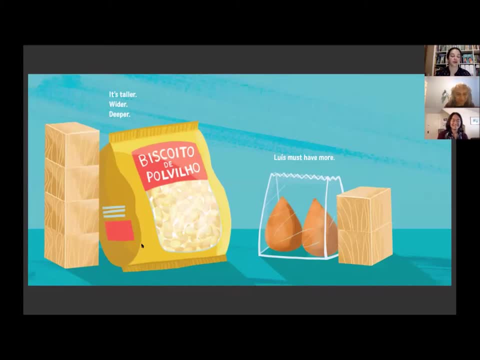 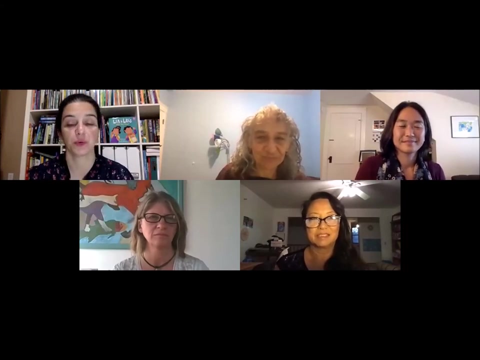 must have more and that's when they're going to um start. uh, you know, trying out several different ways to um, compare both the snacks and uh, come up with a, with an answer. okay, so, um, yeah, branching out, transition from that. marlene and anna, could you tell us a little bit about? 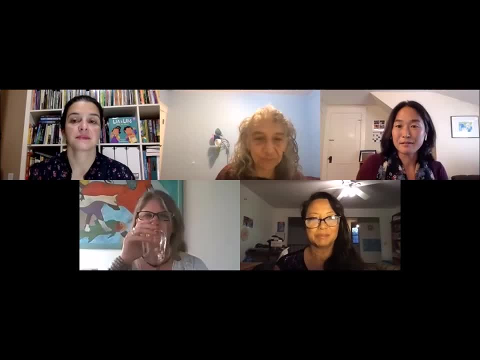 more about the math and the story. so we see that starting to come out in those that part of the stories anna just read. so where is the math and why is it important for young kids? well, lee and louise. explore measurement. the way young children really learn by the hands-on comparison. 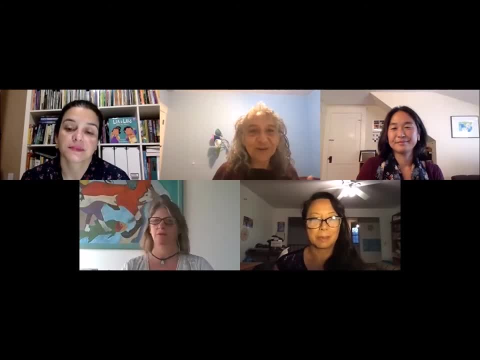 of sizes, amounts and weights and i think the the story does a wonderful job of taking the reader a long with leah and louise and kind of grappling with which is more, how do we compare? in everyday life? comparison and measurement is not a word problem where you're told you must compare pounds. 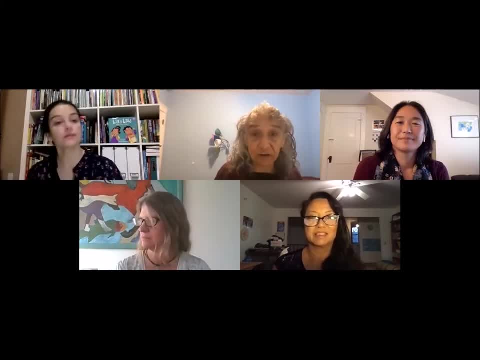 and ounces. you have to take it upon yourself to figure out. how are these things alike? how are they different? what's the best way to make that comparison? and i think that what anna touches on here is math. that's actually important for all ages. a lot of times you see kids in elementary school, or even older, really struggling with 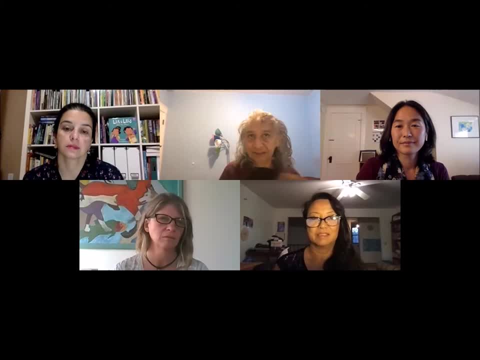 these abstract formulas of: well, how do i convert this measurement into that measurement? they don't know what those things mean. so they may be- may be successful or not successful at working with the abstract notion of pounds and ounces, but they've never had that visceral experience of comparing weights and they've never really talked about. well, why would i? 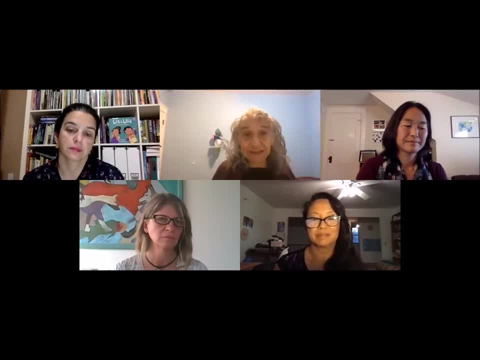 want to compare by weight versus by size or by quantity and um. one thing that i think is interesting to mention is that, um, when i was first writing the story, i was trying to figure out, okay, what is going to be the mathematical plot for this story, or even the plot in general is looking back. 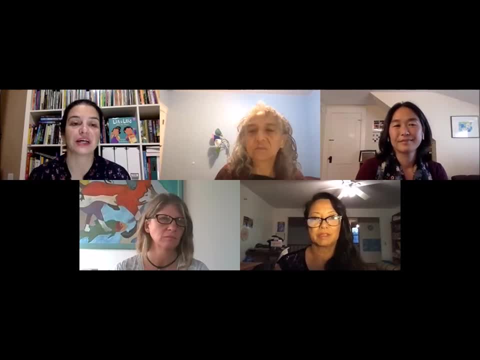 to my culture and everything. and i remember this one question that my parents used to ask me: what weighs more, a kilo of cotton or a kilo of cotton, or what is the mathematical plot for this story lead? and of course they both weigh a kilo, but the point is that a cotton 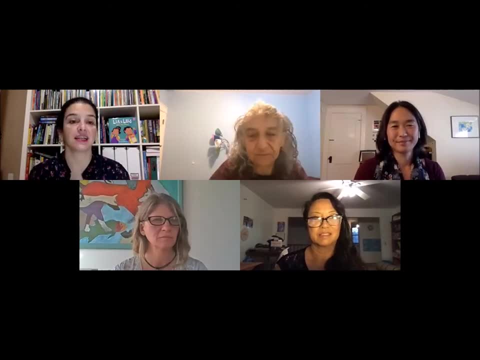 occupies way more space than the lead, and so it's something that, if you look at it, it appears to have. you know it seems to have to have more but it takes so because it takes so much more space. but if you compare the weight, so the weight is not corresponded to what you're looking at, the impressions that 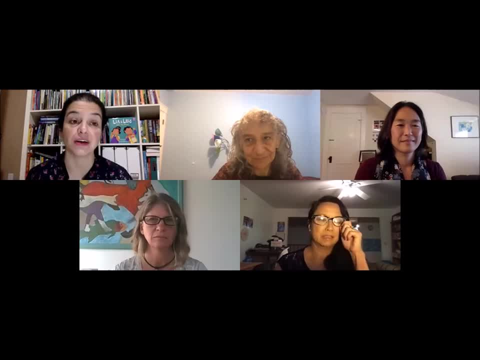 you have, and so. so that's really how the story came about, and then, of course, I substituted the cotton for the Biscoito de Povilho and the lead for the coxinhas, but so that's sort of how the story started and it's sort of a tricky. 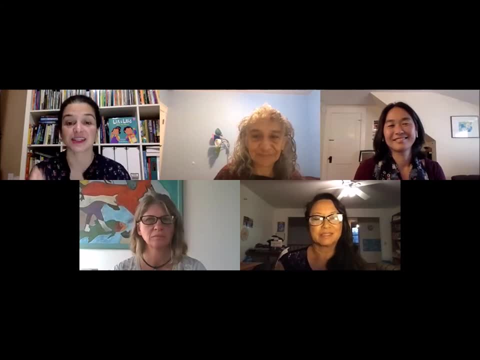 question, even though you're saying a kilo, right, because sometimes, like Marlene said, you don't really understand as a child what what a kilo is. so that was the whole. that's, that's how the story was born, thank you, so so for kids, but what's? 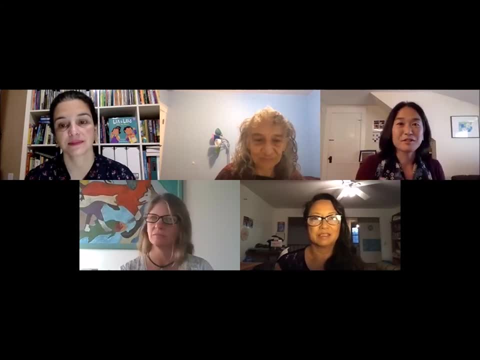 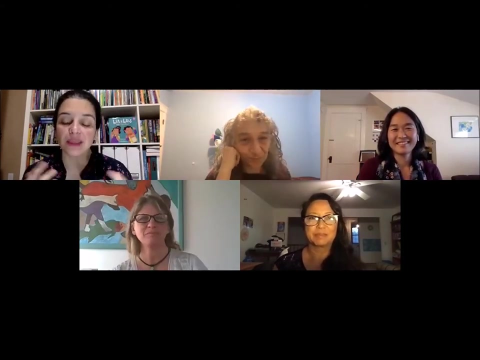 one good activity that I could do with my children to explore the informal measurement in the story. so I'm going to go ahead and go first, Marlene, if you don't mind. yes, I absolutely. um, so one thing that I really like about these stories: the fact 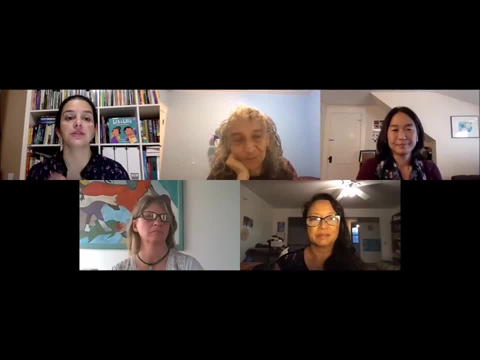 that you can use it anywhere because, as you said, the the the goal of the series of voice to show everyday math. right, so we are always. we there's math all around, we're always doing math and so, even even though we might not realize it, so one 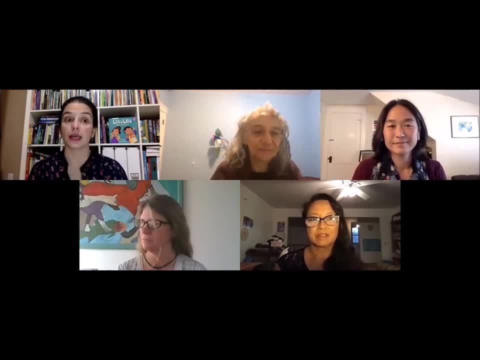 thing I thought about this story was: okay, a, this is something that we can use anywhere. We can go to the grocery store and we can ask the kids: okay, what is heavier? Is it this apple or is it this watermelon? Or, if we can compare things, that something that looks. 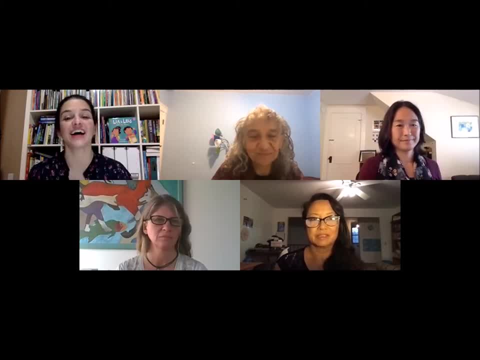 that is bigger but actually weighs less is even better. So that is one activity that you can do anywhere. You can do it at the grocery store, You can do it when you're playing with Lego pieces and wooden blocks. I mean, there's so many ways that you can use it. 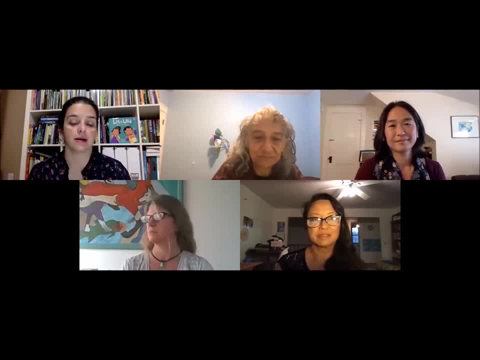 And then, obviously, there are the ways that you can use that book and activities within the classroom to show how to compare and how weight plays a role in it, And I, like I think maybe Marlene would be a better person- to talk about the activity itself. 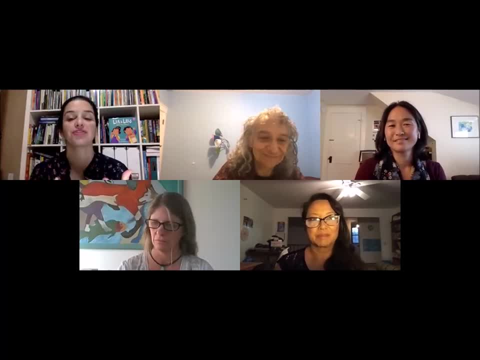 But I like comparing it, I like trying to show the kids that they can just have them make an estimate And just by looking at it, what do you think weighs more? And then actually holding the objects. Okay, now, what weighs more? 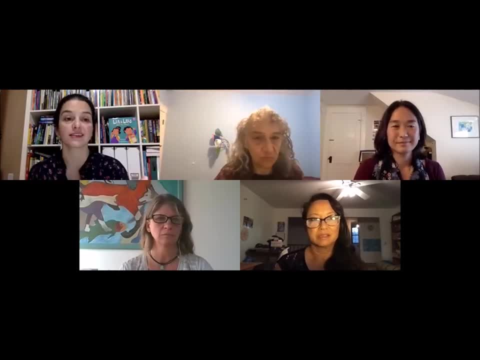 Is it the cotton or is it the rocks, for example? And then if you have a scale that allows you to actually make sure that your estimate was correct or to try out your estimate, that is even better. And eventually, putting the objects in order, adding objects to it. 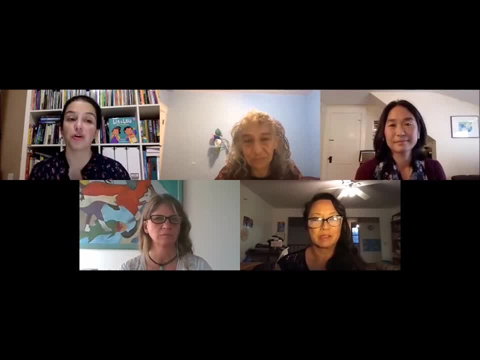 objects that the kids are interested in, the Lego pieces, for instance. I keep thinking of Lego for some reason because we use it so much, But I will let the math expert talk more about it. Okay, I'm just looking around my daughter's room here. 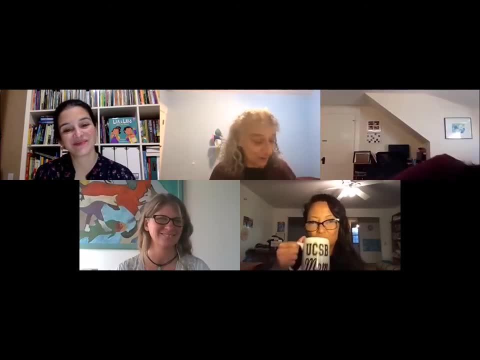 for things to compare, just to show you. I think you kind of covered everything, Anna, But I was just going to say, if you're in a group or you're doing a Zoom story time and there are siblings, encourage them to figure it out together. 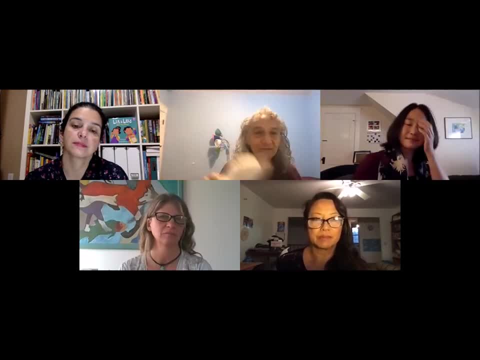 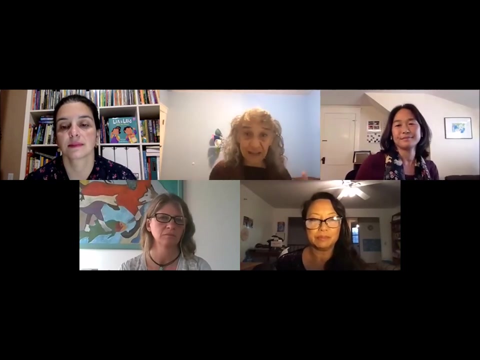 Pick two things. It could be a big ball or a stuffed animal and a phone. Okay, Something in the middle. Have them decide. you know, have them talk about which weighs more. That's going to get them talking together, naturally using weight language. 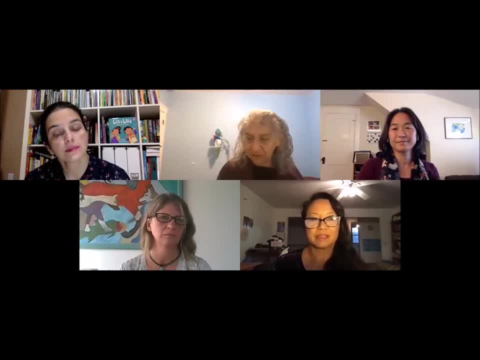 getting that sense of. well, this is heavy. Why is this so heavy when this is so much bigger than this thin little phone? But it's heavy And it kind of sparks thinking about density- You don't need to use that word- with them. 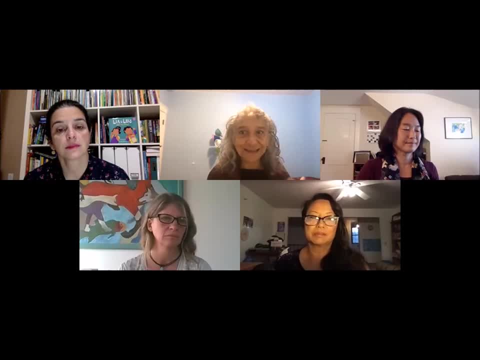 But that's an important concept in math and in science that kids- kids are, you know- really have trouble with in later grades And just using the language about heavy, light, big, small and starting to coordinate those things in their heads at a very young age. 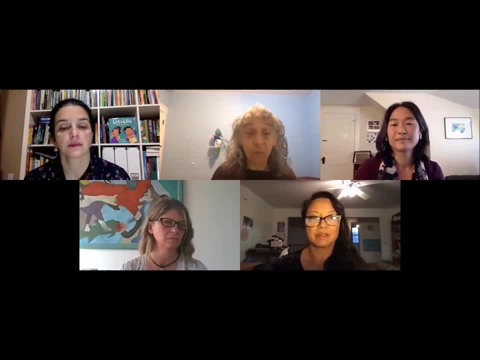 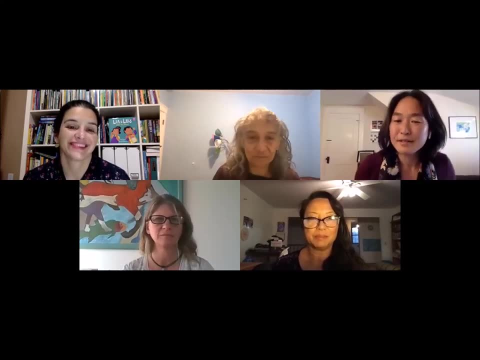 can prepare them for meeting those concepts in a formal way in later years. Thanks, That's great. both of you Thank you, So does anyone. if anyone has any questions for Anna, please put them in the chat And I We can ask some of her. 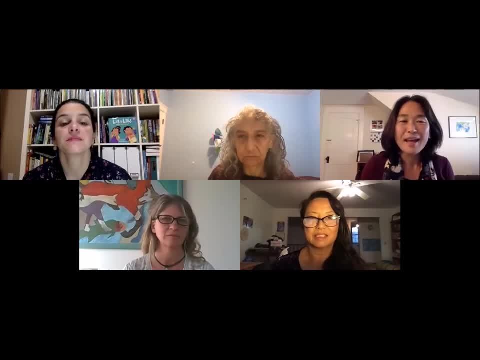 So in the meantime, Anna, I did have one last question for you. I know that we talked about well, are Leah and Louise Brazilian or Brazilian American, And can you talk a little bit about that and how you decided on their identity? 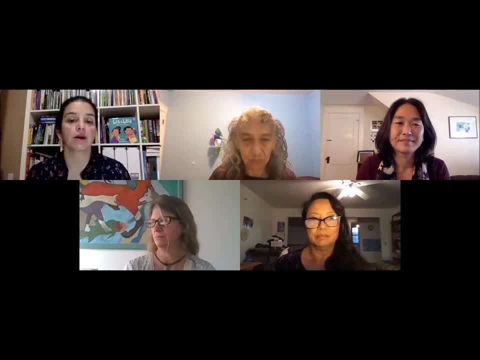 Sure. So when I wrote this story, I thought it could very well be a story set in Brazil. But I kept thinking about it and thinking about the reason for the series and everything, And I decided that they would be Brazilian Americans, And the reason for that is because I wanted any immigrant kid. 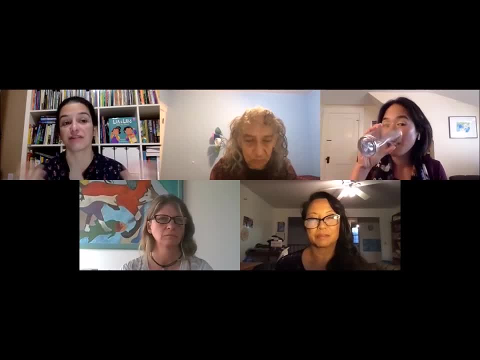 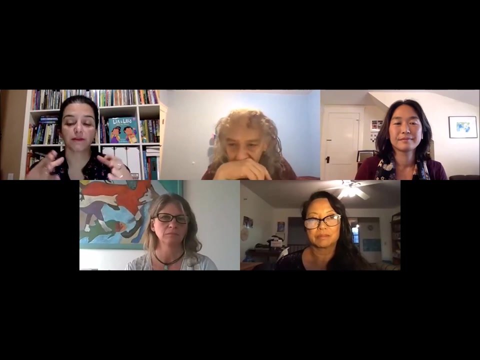 like kids, like my kids, who are the kids of immigrants, first-generation Americans And also any, specifically of course, any Brazilian Americans, to see themselves in the book, but not only to see themselves in the book, to see themselves belonging in the United States. 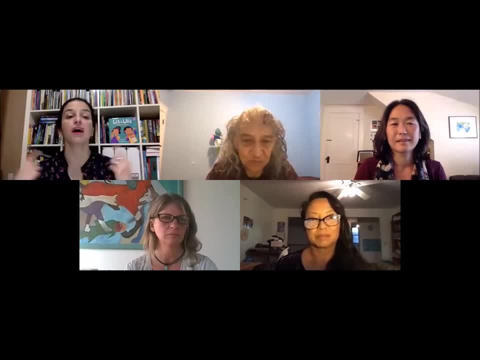 And not only for them, but also for the other kids that are looking and reading this, that are reading the story. I think they should be able to, through this story, be able to see, you know, make an impact on an individual's life and life as a person. 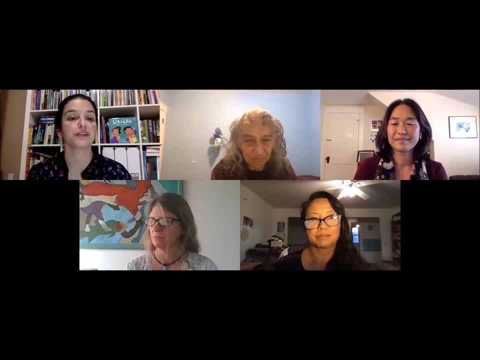 And, uh, leave them with some kind of advancement in them, their own philosophy, And I've also put it all together in the book and it's it's definitely important for us all to take advantage of that and to be more. 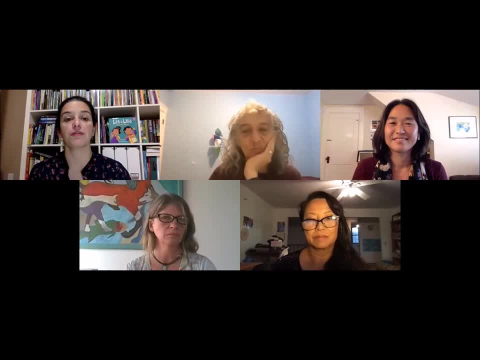 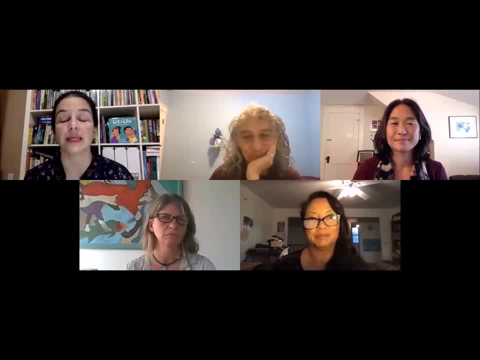 um, um, um, um, um, um. this land so, um, so anyway. so so that was the point of the story and, uh, i hope, i hope kids will notice that i don't know who knows right, but i hope. so i hope it accomplished, thank you. 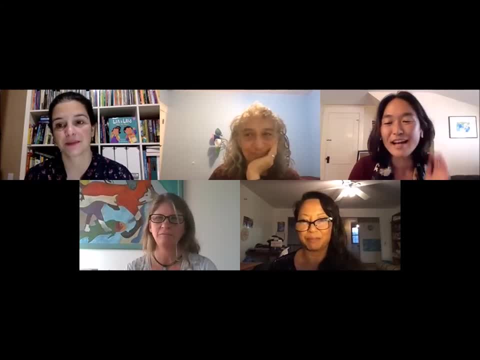 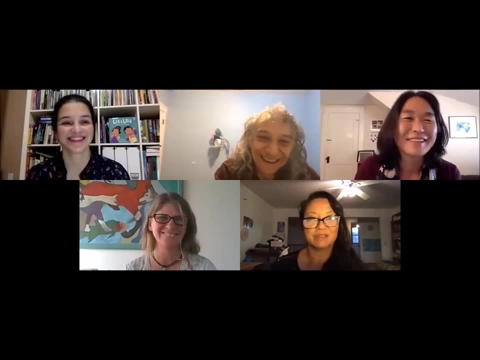 anna. well said, we have some comments in the chat. pamela says i love the story and all the thought that went into it and erin says: hi, anna, are you more like leah leah or louise? i think i'm a little bit of both. i am very competitive, um, especially with my brothers. uh, very competitive. so there is. 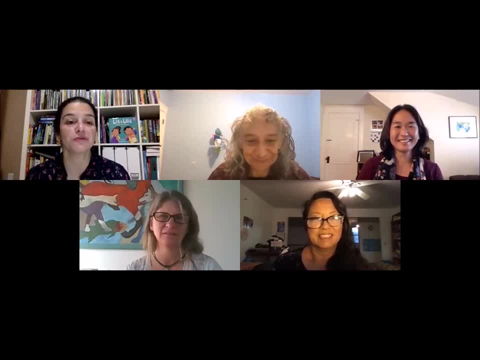 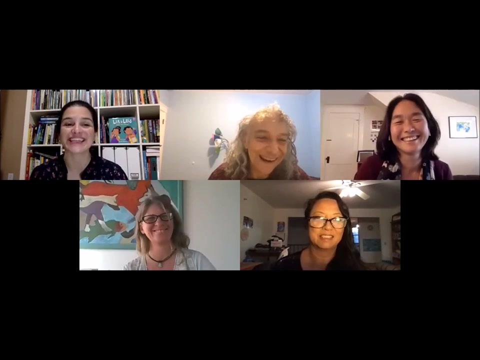 that part of louise in me, but i i'm also very patient, um, when i am doing anything, i have a lot of patience, uh, like when i'm painting, or although i paint. i didn't illustrate the book because my paintings are horrible, but i do paint, um. and so when i'm doing any type of art or or building, 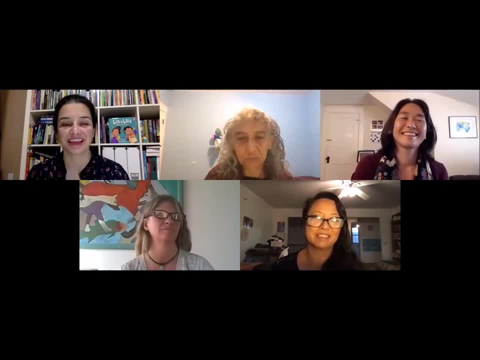 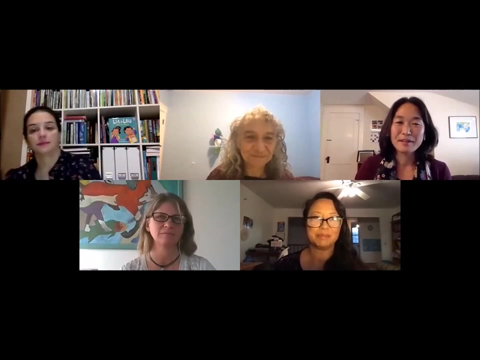 anything. i am very patient, um, so i think i'm a mix of them, the best of best of both worlds. thank you, anna. okay, so if you're just joining us, we are, um in a conversation with the, the creators of storytelling math, and we've been talking with anna crespo, the author of leah and louise, and 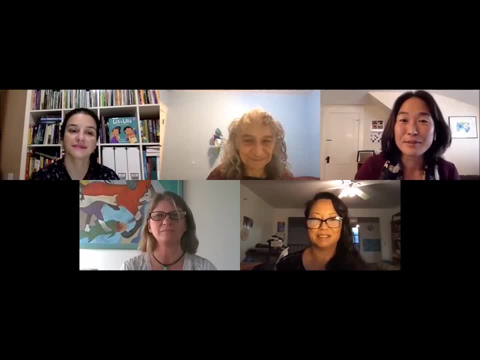 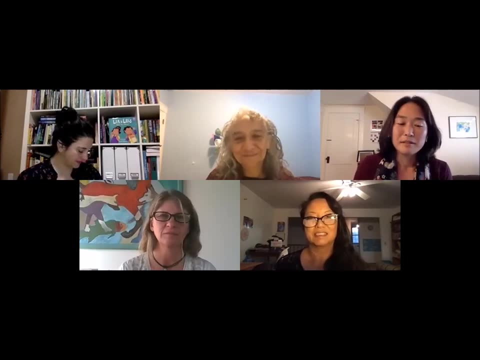 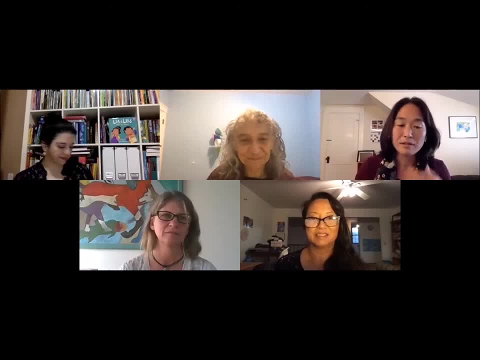 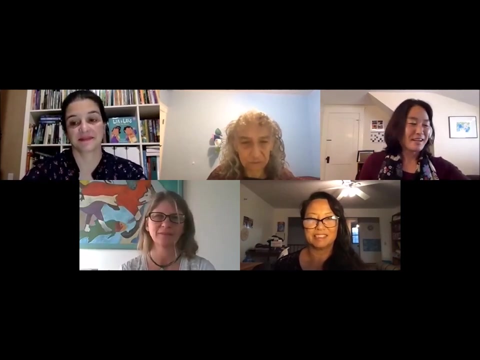 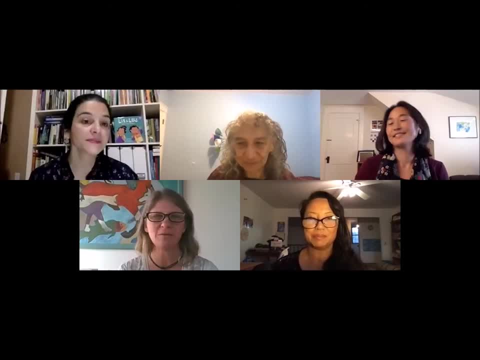 so, sarah, you are a scientist. how did you come to write a book about math? um well, a friend in a writing group friend actually told me about the call submissions and i was kind of curious so i just looked through it and then i realized one of the topics was classification and sorting. 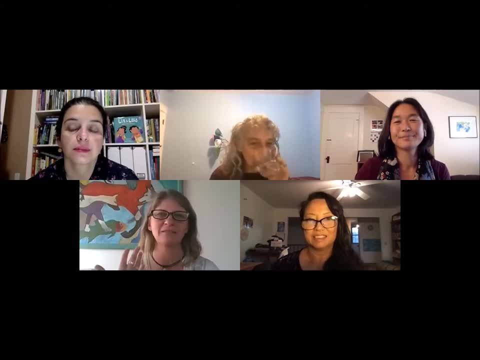 and that's really just a. it's a science topic and a math topic and i thought that's that's a topic that i actually was teaching at the time to undergraduate students, so i thought i'd give it a try and it was a lot of fun. i'm really glad i did great, but yeah, we are too. so what drew? 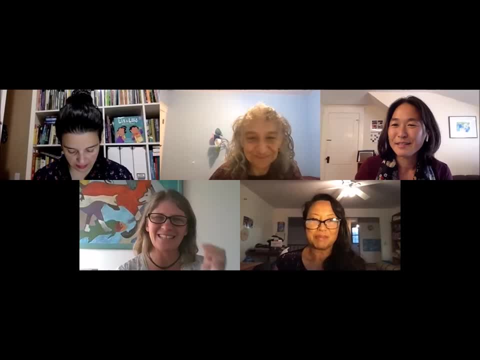 you to start telling math when you read those submission guidelines? wait, say it again. what drew you to start telling math? oh well, i thought, um, the idea of teaching, teaching science or math using a fictional format was very intriguing to me. i think that a lot of times there's this dichotomy between kids who 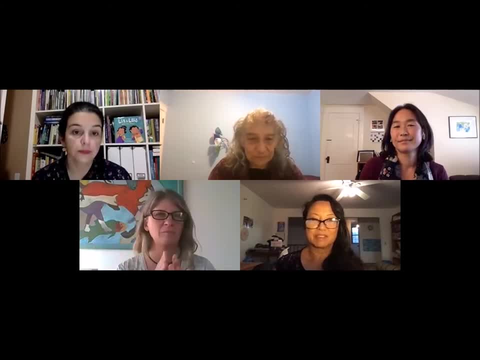 are non-fiction kids and kids who are fiction kids and they get split and really it just needs to come together because it's both. it's a false dichotomy. you know, math and science are part of everyday life and stories are part of everyday life and stories are what um. 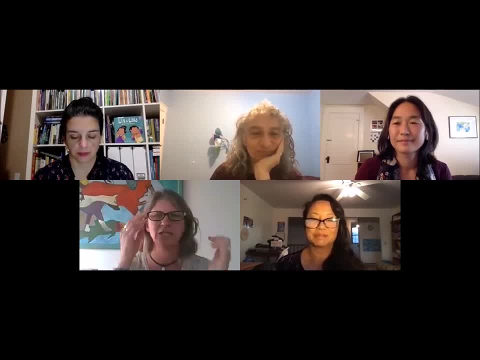 compel people to, you know, to learn, especially certain kinds of kids. so combining the two was important and also just the diversity mission. i think it's just so important for children- um, all kinds of children- to see themselves in books and there's there's really a lack of that and this project was really 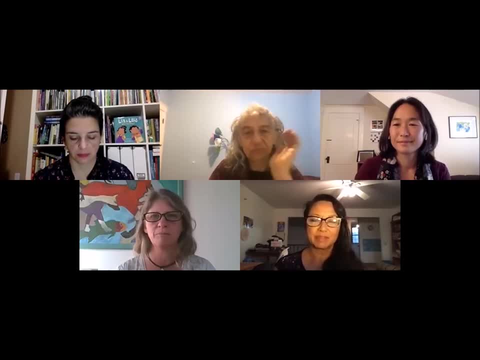 um, addressing that lack. so that was important to me as well. great, thank you, and can so? can you tell us about the animals? would not leave. what's it about? here it is, i'm just going to hold it up for a sec. um, i'll show you a little bit about the animals, but i'll show you a little bit about the books as well. 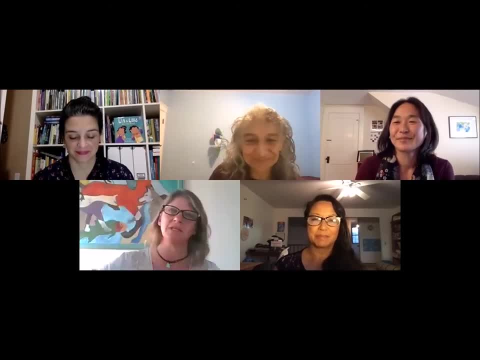 i'll show you the slides after, but just to have a visual. so, um, this is marco and he envisions himself as a scientist and he has a bunch of stuffed animals. his mom tells him to go to sleep and or to clean up his animals before he goes to sleep, and he has this idea that 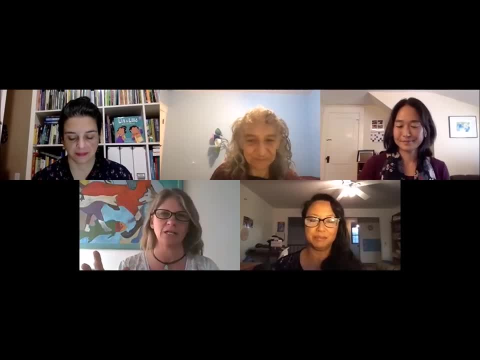 he has three baskets and he's going to sort them into these baskets, um, using different categories. but the animals don't cooperate, their defined definition of you know. he sorts them by size, he sorts them by how they move, he sorts them um um by what they look like, but they keep. 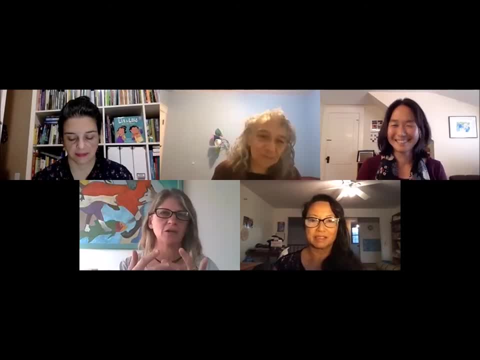 climbing out and complaining because they want to be with other animals that they are closer with, you know, emotionally, and he has to figure out a mathematical solution. um, that works emotionally. so it's, it's a book about empathy, but also about math. so, yeah, should i do you want to read a little bit of it? 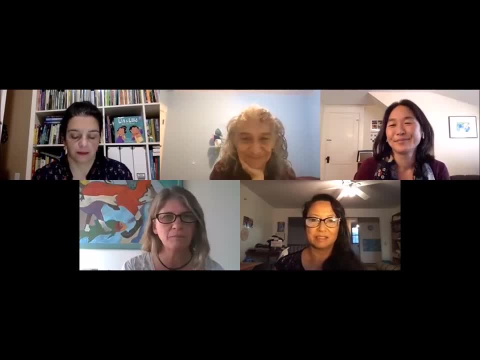 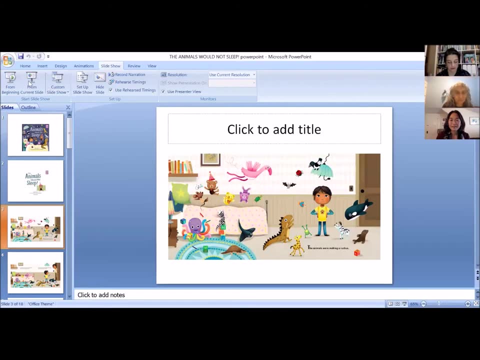 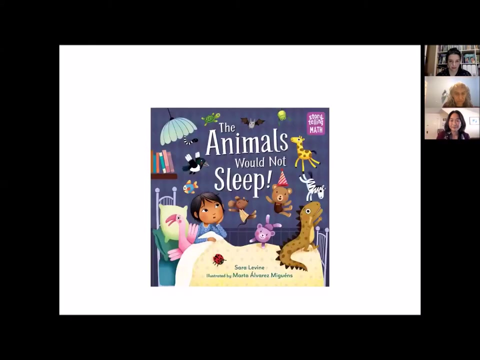 yeah, why don't i go ahead and share that? i think it's actually here we go that work, or is that it looks like it's actually showing? let me see if i can right that looks better. okay, the animals would not sleep by me. and illustrated by malter marta alvarez mcguinns, who did a. 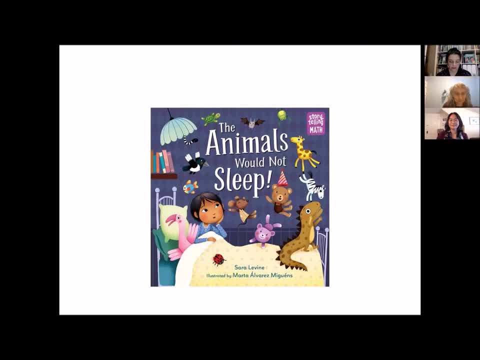 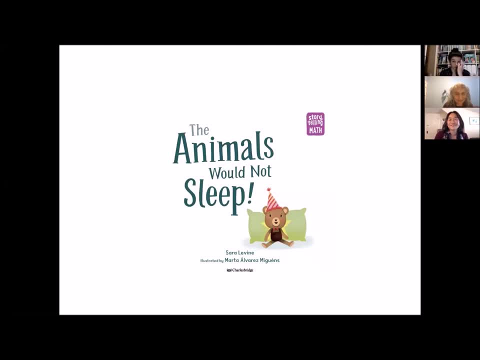 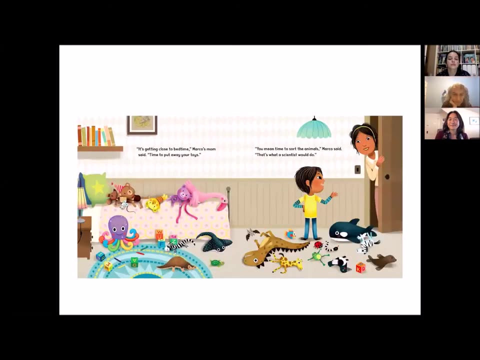 fabulous job. i'm just so thrilled with the book and hoping that at some point when i say this online somewhere, she will hear me. okay, the animals working a ruckus. it's getting close to bedtime. marcos mom said: time to put away your toys. you mean time to sort the animals. marco said that's what a. 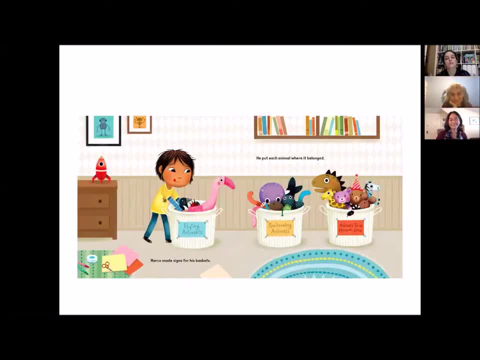 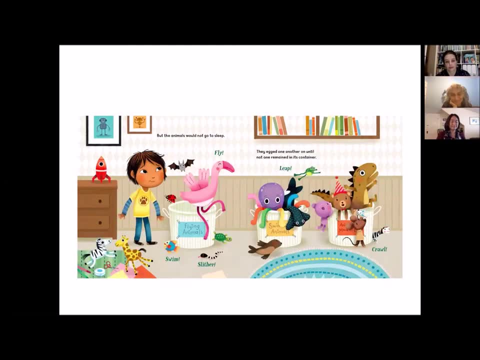 scientist would do. marco made signs for his baskets. he put each animal where it belonged, but the animals would not go to sleep. they egged one another on until not one can remained in its container. perhaps they weren't tired enough yet. marco gave them a little more time to get their 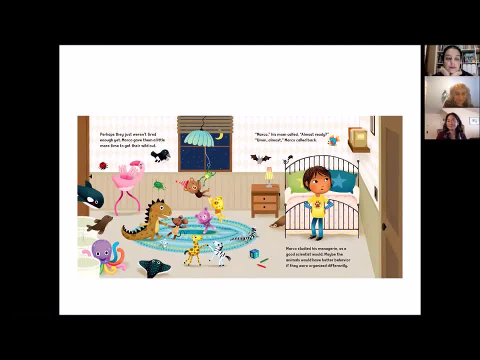 wild out marco. his mom called almost ready, um, almost. marco called back. marco studied his menagerie, as a good scientist would. maybe the animals would behave better if they were organized differently, and i think that's a good taste. should i keep going, or is that good? um, that's good why. 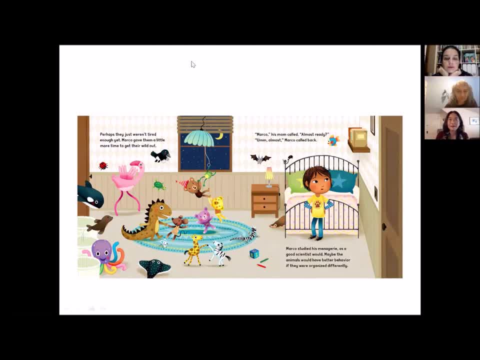 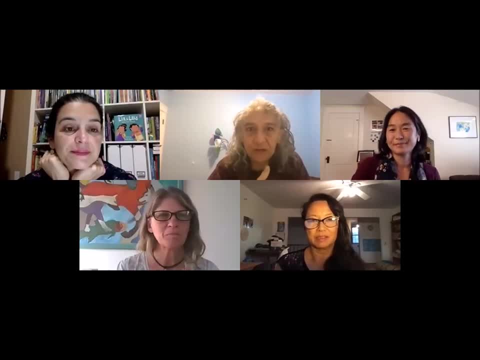 don't. can you and marlene uh talk with us about the math? i mean, what is the math? where is it and why is it important? do you want me to go, or sarah? um, yeah, why don't you go ahead and start, marlene? sure, so, yeah, so the math. 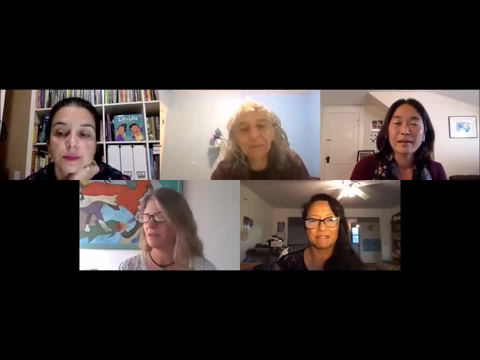 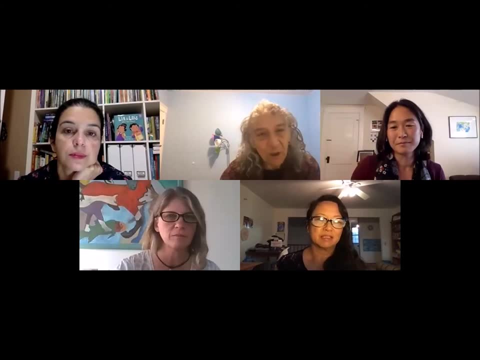 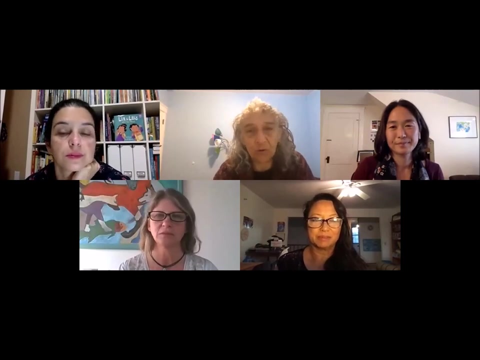 involves sorting, classifying, where he's combining mathematical thinking and empathy as he looks at different ways to group his animals so that they're all happy. and we often think of sorting as something that very, very young children do when they kind of stop when they go to school. you know, the red things go here and the blue things go there, um. 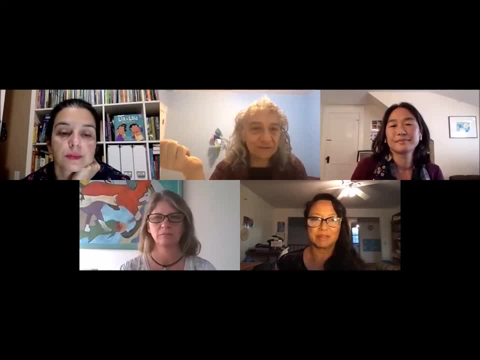 and but yet sorting and challenging is really fundamental for understanding um data science and statistics. it kind of comes back in a big way in the end of elementary school, and one of the things that kids really need to understand um- and they often don't when they're very young- is: you can. 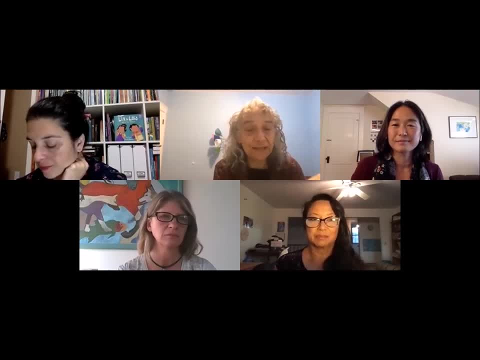 take the same set of things and sort them in different ways. so he sorts his animals by color, but and then he puts them back together again and sorts them the day after the seventh grade. um, and these are not academic four school years, and it wasn't even a year before him. can i use these teaching? skills and idea skills. they interact with the teachers and they interact with the numbers. every week there is something aboutивать science. you know we be a group of kids in our day of work that has very much primary suggestions and made up our rebuild in our bloss. Kafka нельзя to be involved. too simple, because i always knew: do what we need to do. that. 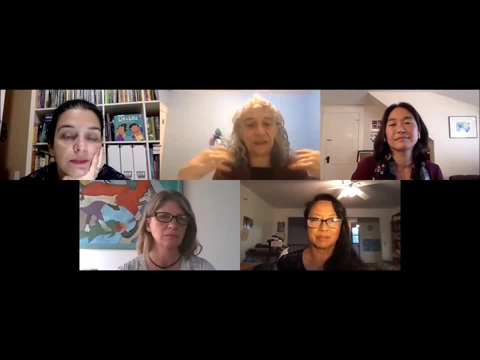 them back together again and sorts them by method of locomotion and then he sorts them by size. i think i have the order of how he does it wrong, but you know, but he but he breaks them into different groups and and that's kind of an abstract concept. it's used in data science, just statistics. so we 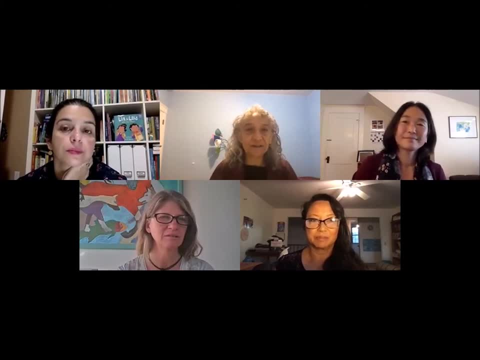 look at, you know, how does presidential preference break down by gender? and then we look at how does it break down by state, and then we look at how does it break down by age or geographic region. that's that very flexible mathematical thinking which we are starting to see marco use as he groups. 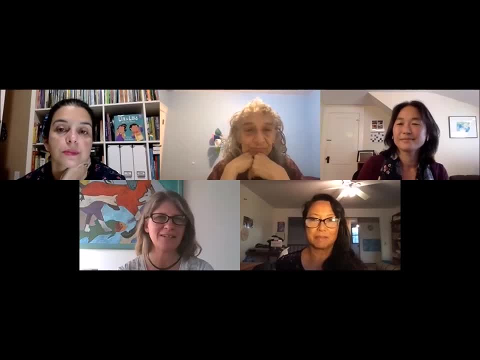 his animals different ways. that was fascinating to hear you talk about. i'm so glad we did this, yeah, okay. so, um, what are some activities that i could do with my kids to explore? all that great math and animals would not sleep, so one of the things. um, i think there's two, two main ways to go about. 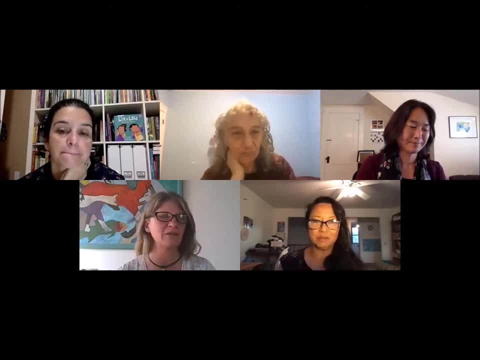 it. and one of the things: um, i think there's two, two main ways to go about it. and one of the things, um, i think there's two, two main ways to go about it. and one way is, you know, gather, a bunch of gather, a bunch of items, um, in your house or your school, um, it could be stuffed animals and you can. 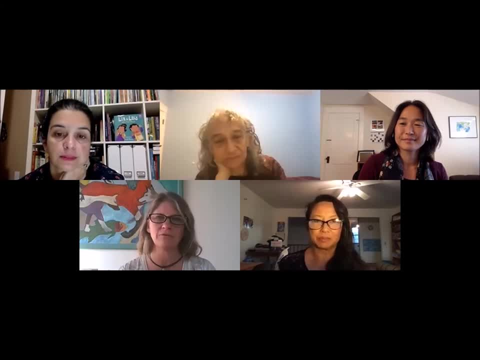 make the same categories that marco made, or you can have the kids come up with different categories and then group them um. another way to do it is to just gather a bunch of random objects in the house. you know, get get everything in the junk drawer and put it down, or gather things from 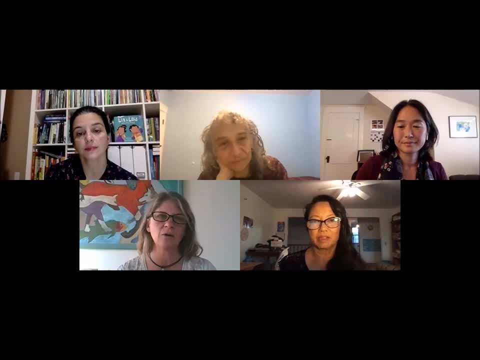 nature and um. have the kids make up their own categories and sort them, and then have the parent addle, involve, guess what the categories are, because it's a more creative way to flip it around, um, and also engaging for the adult as well. um, anyway, those are some thoughts. 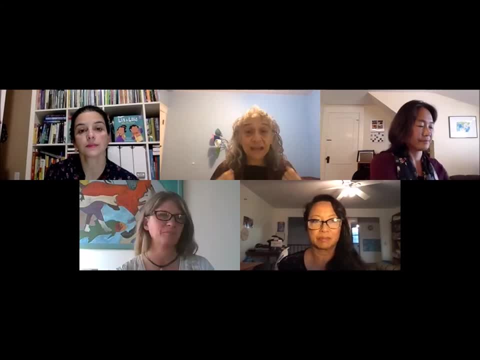 those are great, and i would just add that, as you're doing it, keep talking to the kids, get them to talk about. why did you put these together? there's no right or wrong in this kind of thing. it's. what's important is their thinking, their ability to talk about what this group has. 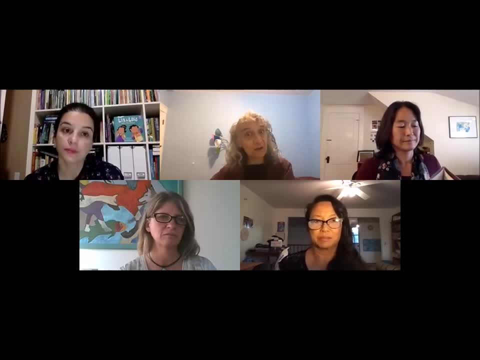 in common and what that group has in common. so the categories they choose may seem kind of strange to you, but if it being able to think through why do these go together and why do these other ones go together is an important kind of abstract thinking tool that young kids can start to develop. 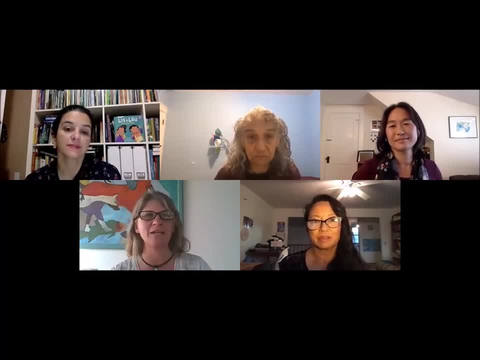 you know, marlene, hearing you talk about that is remind. this is ridiculous, but it's reminding me of when i was in kindergarten. i had kind of a bad experience. we were collecting leaves and we were supposed to put them in categories. the leaves either look like this one or like this. we had to put them where they looked the most. there were three. 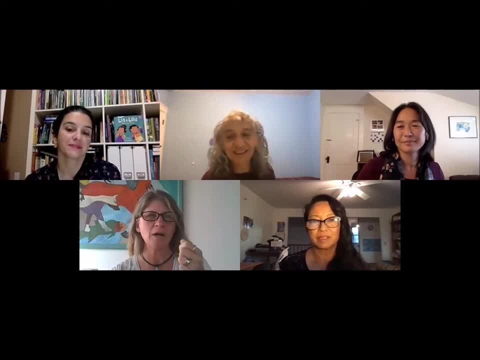 different categories of leaves and i found this leaf and i said: well, it goes in this category because it has rounded edges, and it goes in this category because i can't remember what the other thing was- maybe the color- and the teacher said: no, you have to pick one. at which point i started. 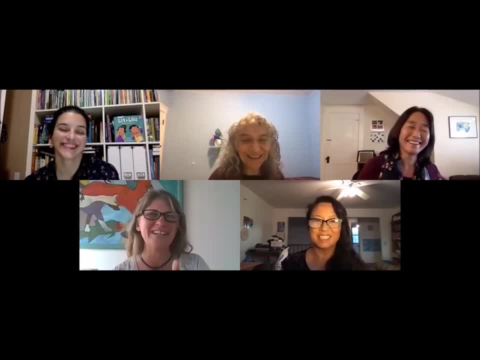 crying because i was four but she was obviously wrong. so the talking about why you pick the categories, you know, i'm remembering it because i was so upset, because i was so shy and i was putting myself out there. i was answering the leaf question anyway, um. so don't be like her, be like marlene talk. 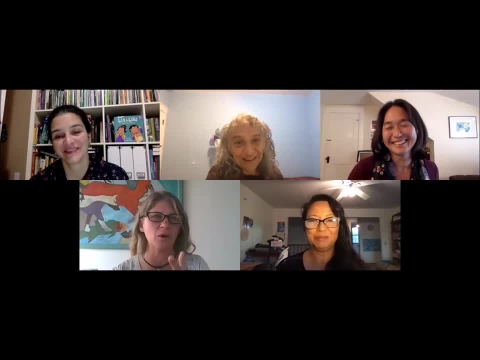 to the kids about. you know why you could fit in different categories and why you know that there's not one right answer in math. well, and there there's an example. my, my kids, who are all grown up now, used to love to collect little plastic dinosaur figures and um, they always made up stories about. 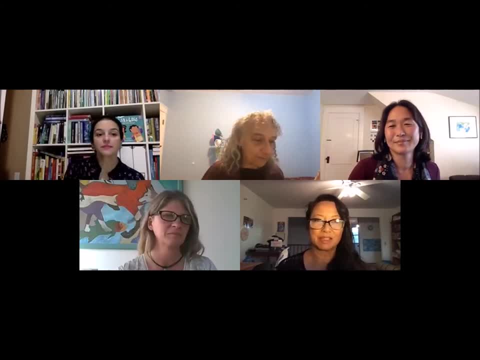 as a natural part of their, you know, setting them up around their rooms. they would make up stories and they would put them in groups. but, um, they used to, the dinosaurs used to go places, so they always had some kind of- whether it was a real vehicle or a pretend. you know this, this piece. 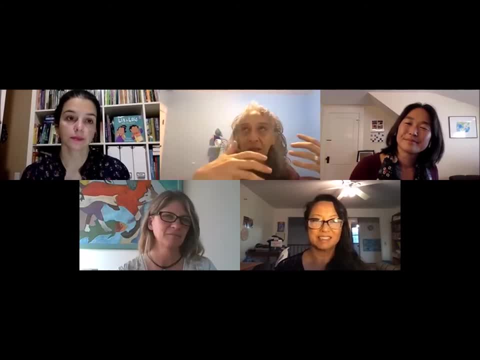 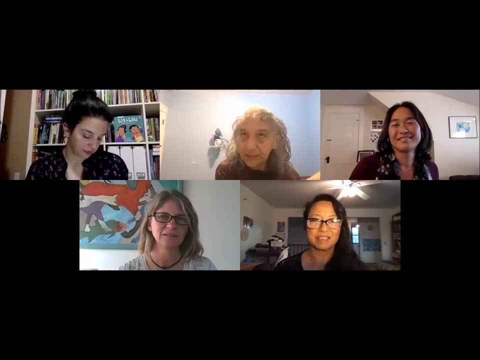 of plastic is a car or a spaceship. so they always had ways to go places and they always had food in their little groups. so they weren't sorting them according to you know what, what period, what paleontological period they lived in or what type of dinosaur they were. 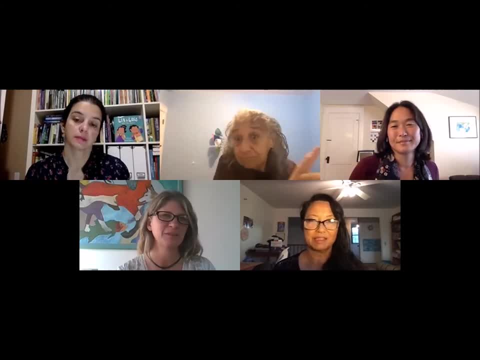 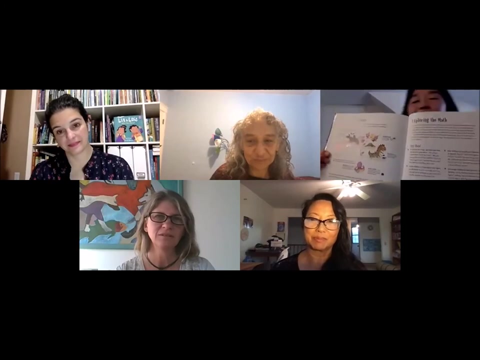 making little sets and that made sense to them. yeah and um, you know the important things that could explain why, yeah, those conversations are so important. at the back of every storytelling math book, we have um ideas. well, there's, there's more about the math in the story, and then there are 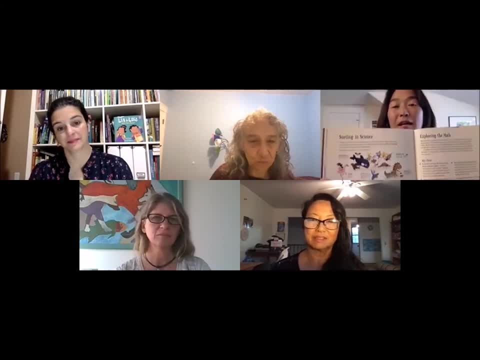 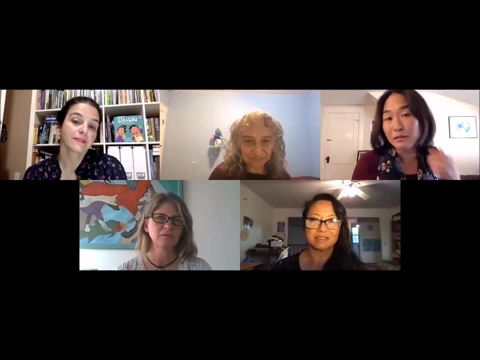 ideas for activities that you can do with the children in your life and in your life and questions you can ask them and we have um downloadable, additional downloadable activities on our storytelling math page on the charles bridge website. so, sarah, i did have one question for you about empathy. so at the end of the book, marco uses. 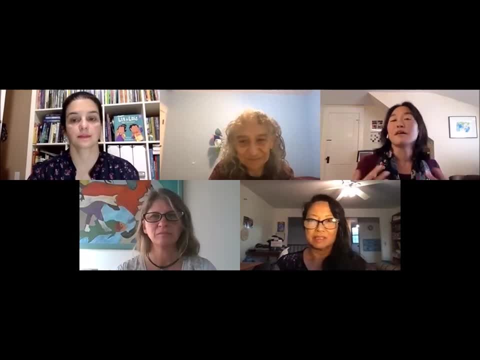 empathy. um, as well as sorting smarts to solve the problem, make sure his animals are comfy. and oh, what prompted you to give empathy a role in the story? well, what's really more important than empathy and kindness? i mean in any book? if i could stick that in there, i would stick it in there. but 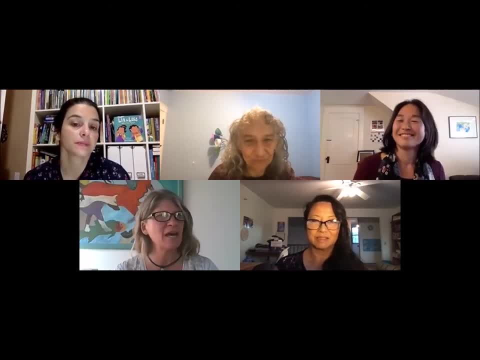 this one in particular. i think that a lot of kids that are young, who are very interested in animals, are highly empathetic and sometimes in the school system those kids get weeded out of the science classes because in order to do well in science, you have to. 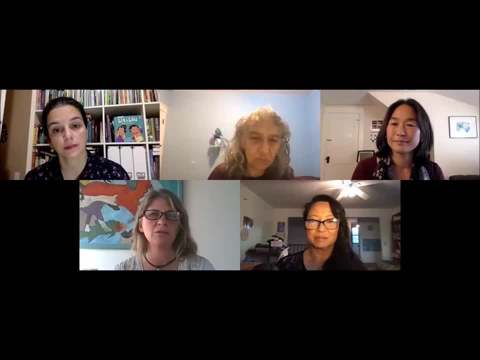 the way it's taught. now you have to a little bit close down some of that empathy to do some of the things that our kids are called on to do. so i wanted to. i guess i just wanted to show a character where, um, he considered us himself a scientist, but also his empathy was up front. so it just seems 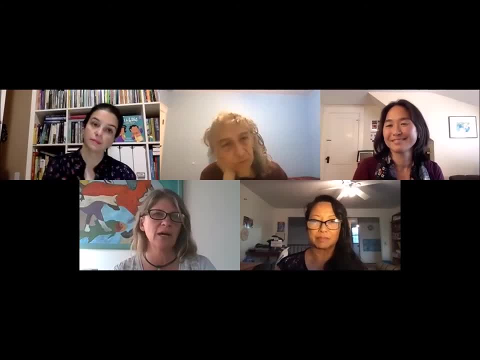 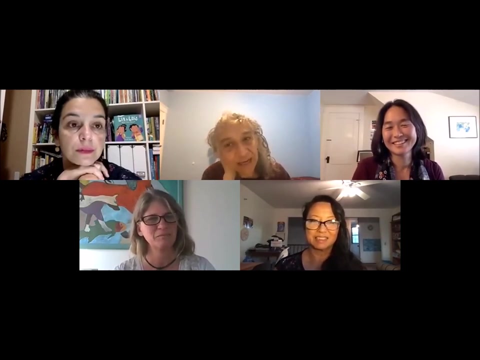 it's maybe my subtle way of starting the conversation about that or or participating in conversation, just really, the way that, um, we see science and teach science really needs to change, and it's totally true about math too. yeah, that's one of the things we loved about this story is that in a lot of 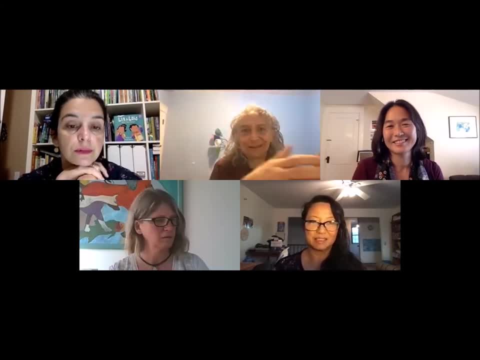 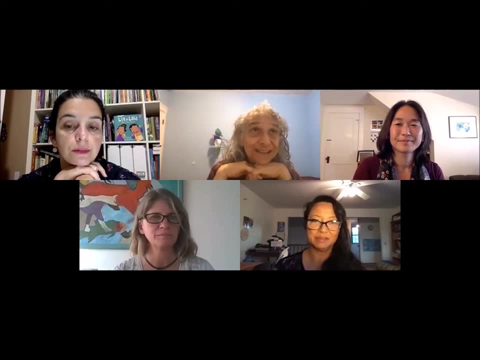 picture books out there that involve math. it's sort of like there's this answer that comes up, it's the math answer and you go with it and the story's over. but here it's it i. i feel like it's more akin to the way we use math in our lives, where 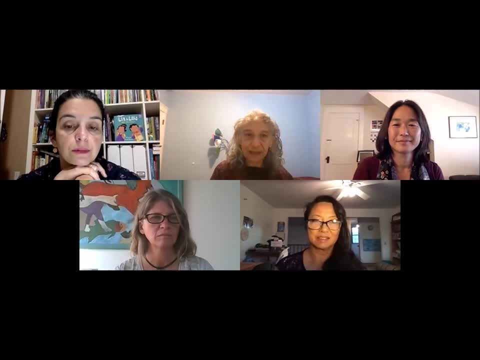 math is one tool to help figure something out, but it may not lead to the answer we ultimately choose, because there are so many social and emotional factors in our lives. um, you know, life is not a word problem, it's you. you put lots of things together when you. 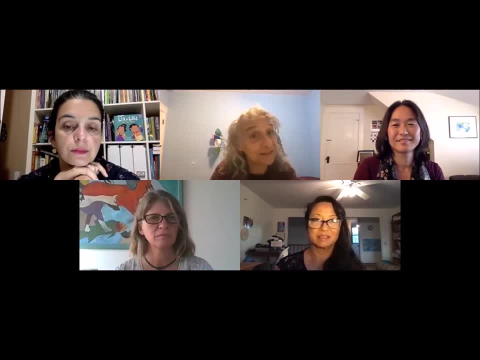 make a decision and math can be a great part of that, but it's not the only part. yeah, i love that, marley. i i would say that all three of your books- anna, sarah and natasha- do have that emotional um component, emotional intelligence component, and the kids, the characters in the book, do use empathy. 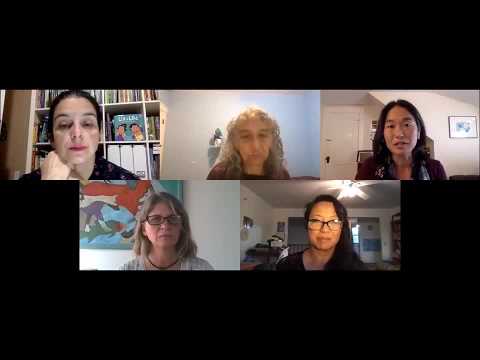 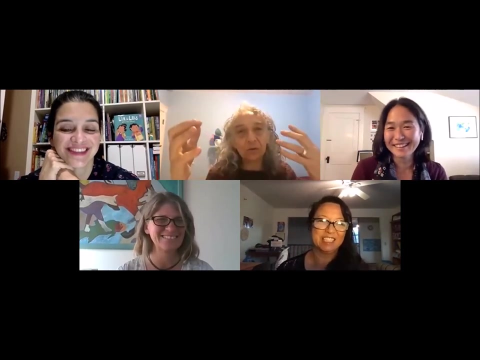 as well as mathematical thinking to come to a solution. and we just love that. marlene, i'm gonna- i'm gonna make a t-shirt that says storytelling, math, life is not a word problem. that's certainly true. that's great. well, i think it also helps kids. um, you know, most math anxiety is. 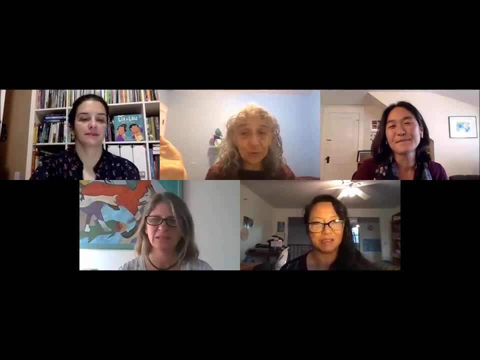 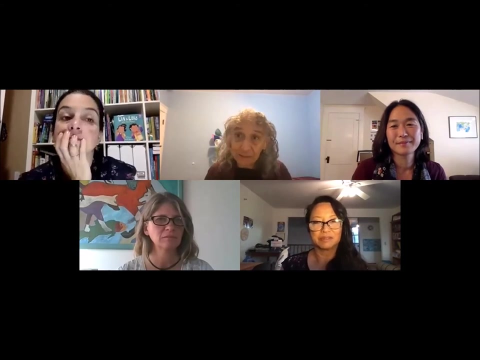 everywhere and it helps kids who don't necessarily see themselves as i'm. i love math, i'm going to go into math and we don't need that because that's a little bit too difficult. it's okay to make a good everybody to think that way, but we do really want well-rounded kids and adults to feel like math. 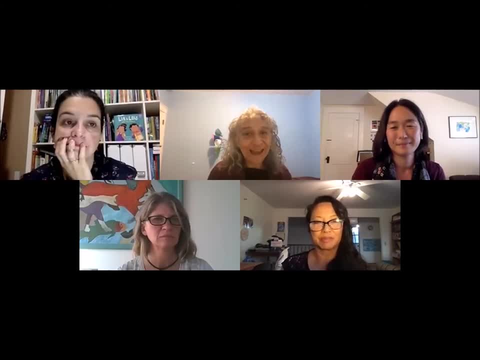 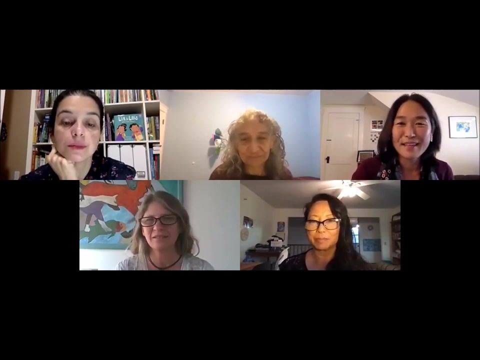 is fine. I'm comfortable with math and by showing it in recognizable context with relatable characters, then you can feel that kind of connection to math. you don't feel that connection if your characters have no emotional. you know trajectory, Thank you. so Erin says: love the use of empathy in these books. Thank you, Erin, we do too. 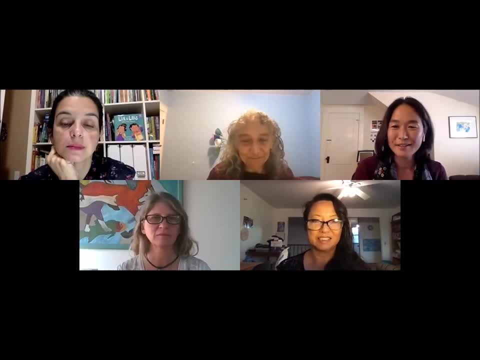 Does anyone else have any questions or comments for Sarah? Okay, so if you're just joining us, we are chatting with the creators of Storytelling Math, and we've talked with Anna Kreshel about her book Leah and Louise, who has more, and Sarah Levine. 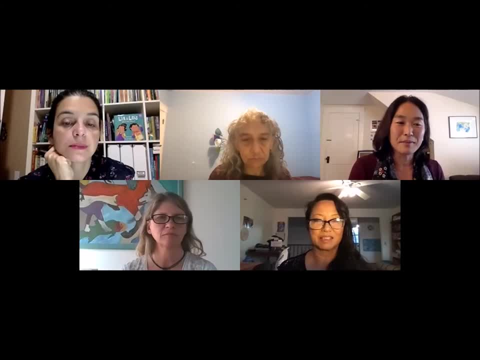 about her book The Storytelling Math, Thank you. We've talked about her book The Animals Would Not Sleep, and now we're going to be talking with Natasha Yim, the author of Luna's Yum Yum Dim Sum. So, Luna, let's see. Natasha was born in Malaysia. 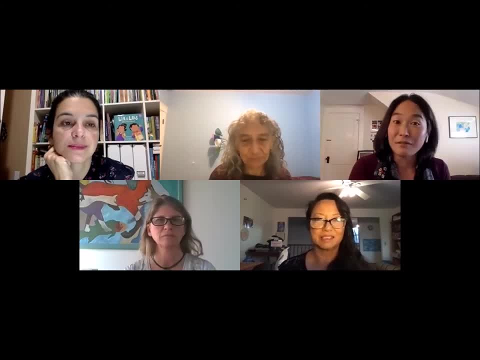 grew up in Singapore and Hong Kong and now lives in California. She is the author of many wonderful picture books, including Goldie Luck and the Three Pandas, and that was our first book together- The Rock Maiden and Mulan's New Year. 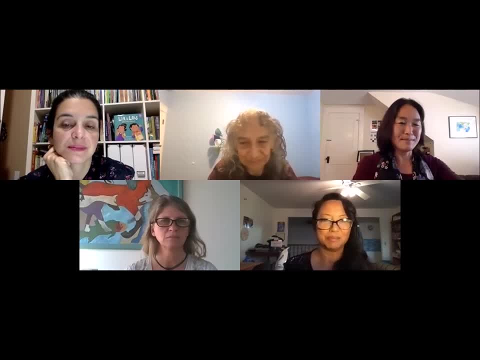 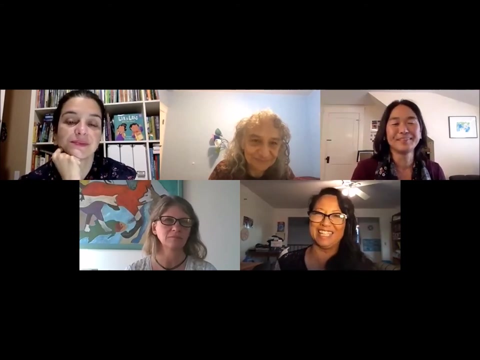 And now she is the author of Luna's Yum Yum Dim Sum. So, Natasha, let me pull up my questions. Okay, so what crossed your mind when I invited you to submit a math story to the series? So the first thing that crossed my mind was: I can't do math, which is why this series is so. 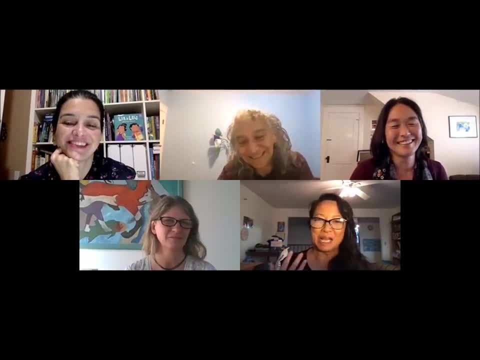 wonderful- just going back to what Marlene was saying and what um Sarah shared- is it's because math for me, growing up and in growing up in Asia, where math learning is very much by rote, so it's a lot of you know worksheets, it's memorization. 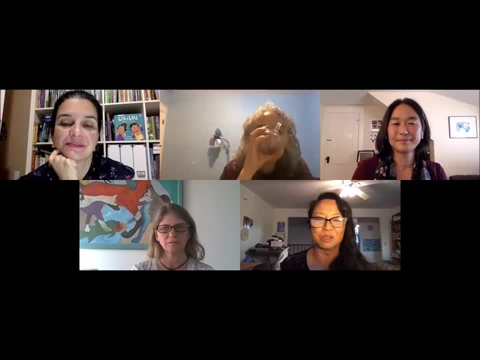 especially in my generation. It might be a little different now, but um, it was worksheets, it was memorizing formulas, it was so and I've always felt, um, intimidated by math and that math. uh, I always felt significantly math challenged. And I don't know if you guys remember the old 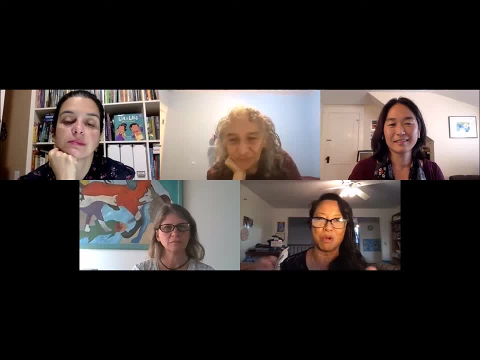 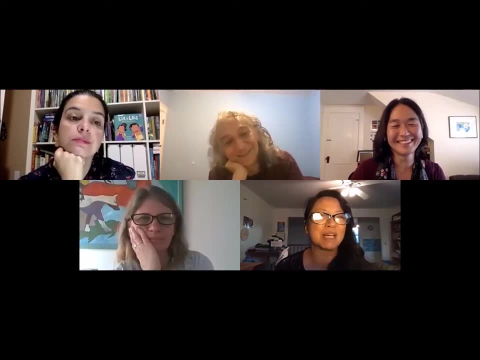 the Charlie Brown movies where the adults were all going wah, wah, wah, wah, wah. that was what it sounded like to me when people talked math to me, And so, um, so I I think the series is just wonderful because of that, because it's true that math is all around us, It's in everyday. 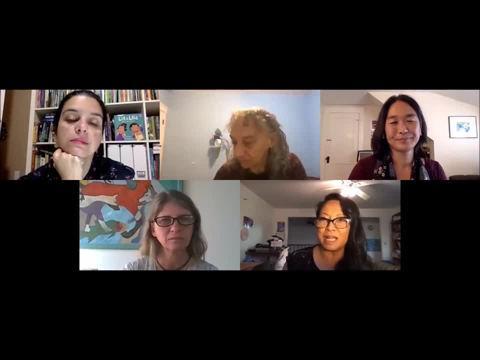 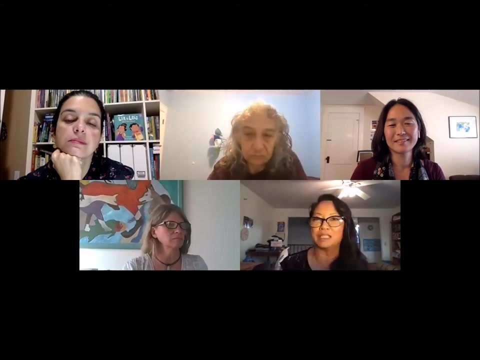 in our everyday lives. except I never saw it that way as a child, You know, math was just a subject in school. Math was, you know, learning all these like different formulas and trying to, you know, figure out things on a piece of paper. Um, so it was never incorporated into. 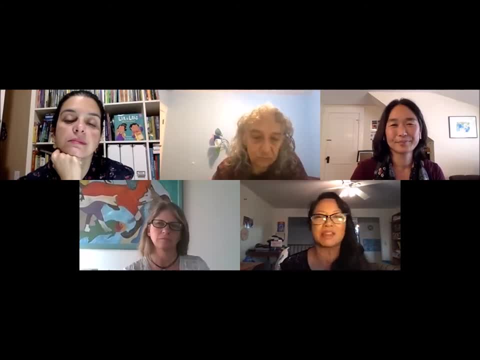 daily life for me. So uh, so I think I've always grown up with that. you know that fear of math and the intimidation and I and I think these stories are wonderful that they can open up math and you can start introducing them to kids at a very young age. 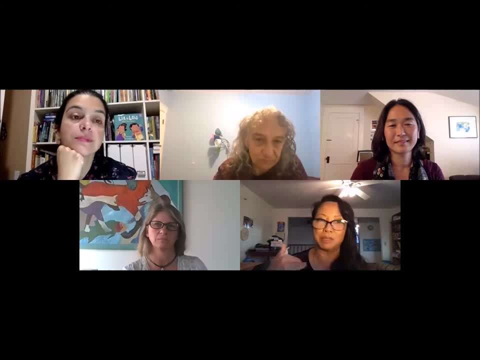 To introduce them to the concepts of math without having it be, you know, um like with uh Luna's Yum Yum Dim Sum. basically, they're doing fractions, but you're not. you know the word fraction doesn't. 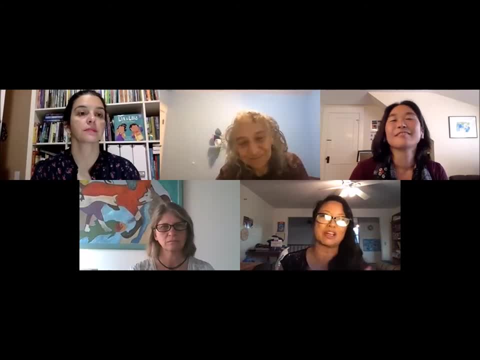 come up, and you're not talking about it in terms of fractions. You're talking about it in terms of: you know how do you share things equitably? So, um, I think that's the the, you know the. 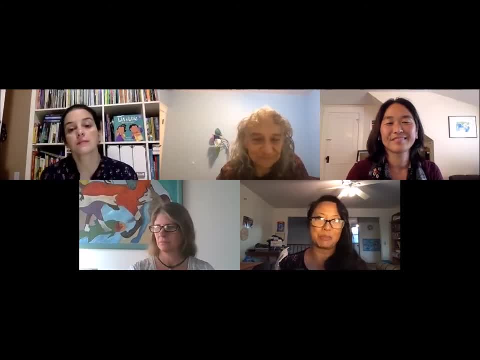 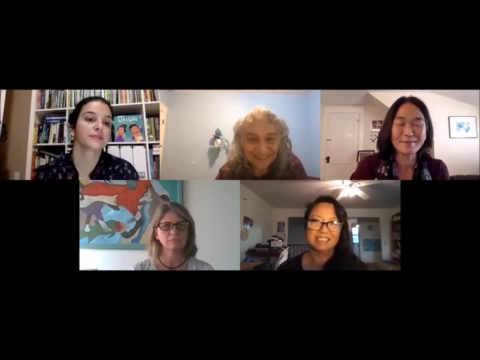 very appealing thing, uh, about this project. uh, to me We're so glad you, you submitted the story and it was we, we were just we were like wow, this is, she's so much fun and uh, I mean we, we enjoyed it so much. So could you tell us a little bit? 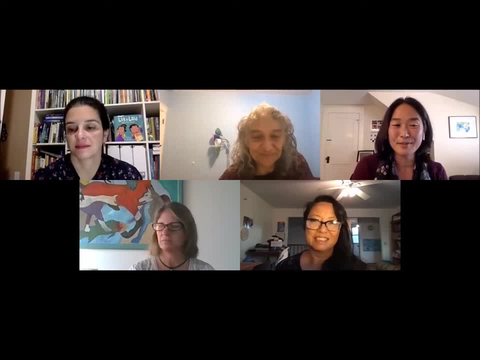 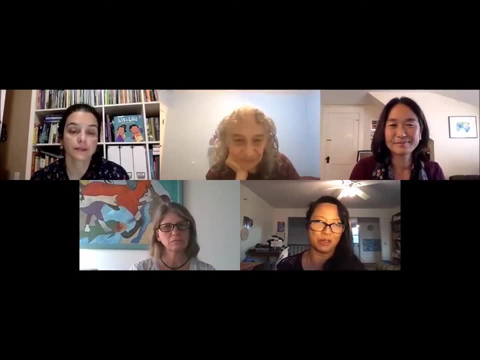 about the story and the characters and then maybe read a little bit of the book. Yeah, sure, Um. so you know, I was uh really interested, uh, you know, um, Anna, when I heard you talk about how you wrote the story first and then you debated the setting um later, that sort. 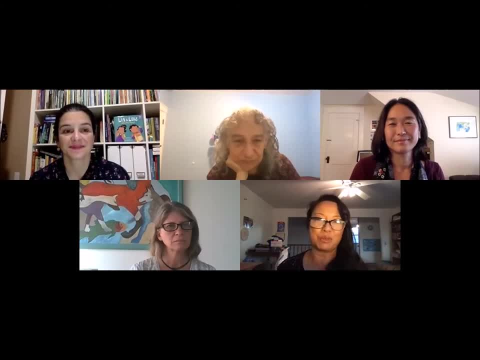 of thing- and for me it was always the setting- came first. When um Alyssa approached me with a story, immediately I thought of having it in a dim sum restaurant, and I think part of it was because, um, I love dim sum, and so the research was really fun because I got to go, you know. 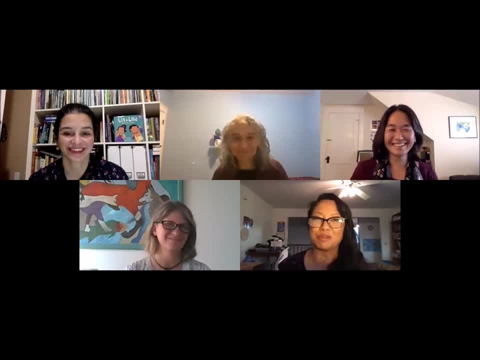 go to, because I don't. I, I live in a small town about two hours north of San Francisco, so all the restaurants are about. the dim sum restaurants are about, you know, two hours away from me, um, but you know I have family in the San Francisco Bay Area, so every time you know, I went. 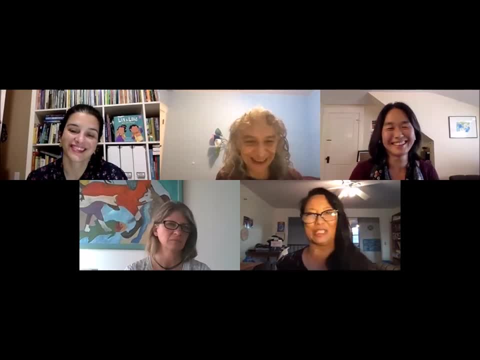 to visit. it's like we got to go have dim sum because I got to do research on this book and it was, um, and my first draft. this, this actually was my- uh, the second draft I had submitted. 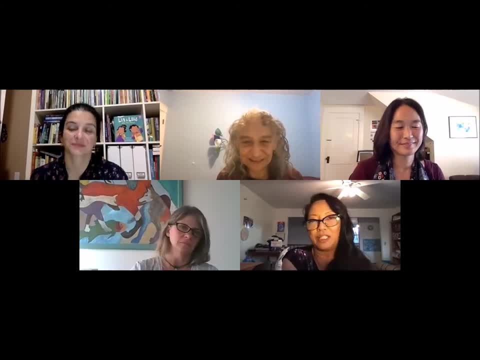 and of course, we did a lot of revisions on it, but the first draft actually was um, about, uh, the the kids eating different kinds, ordering different kinds of dim sum dishes. because the the one thing I thought, the one reason I thought about dim sum was because dim sum 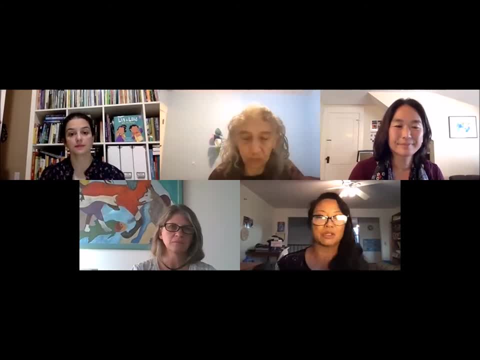 comes in um very different shapes, you know, so that you have, uh, circles and you have pyramids, and you have squares and rectangles, and so I thought, oh, this would be really fun, and then you can kind of incorporate the math, because you're ordering more food and then you're eating. 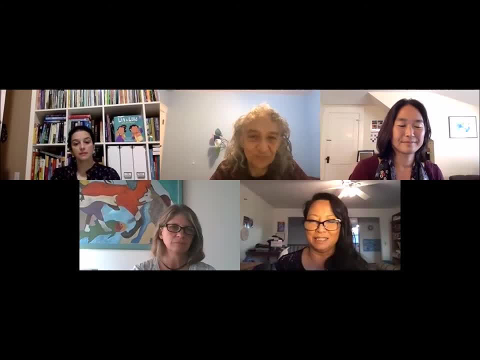 it and you're taking it away. and then I submitted that and, uh, Alyssa was very nice and she said, oh, I love the setting, but we're not really looking for counting or shape book, and so it was back to the drawing board and and then, and to Marlene, thank you. 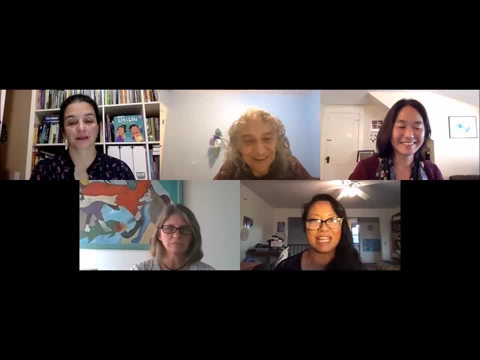 so much for helping me. you know brainstorm, some math ideas and um. so we we finally settled on: how about you know um? how about sharing? you know what? how how can we share? like food. 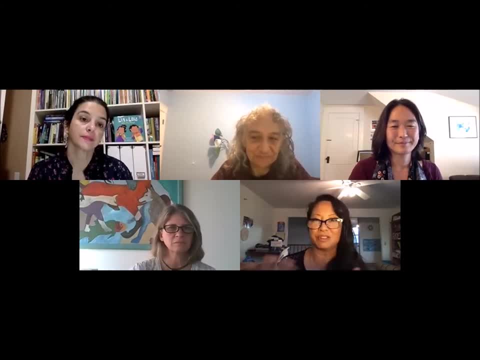 equitably. and then we had some interesting discussions. um, like I think Alyssa and I, you had a discussion and I had a discussion about: okay, what kind of dim sum should is the most you know? should we share? should we share something that or feature something that is? 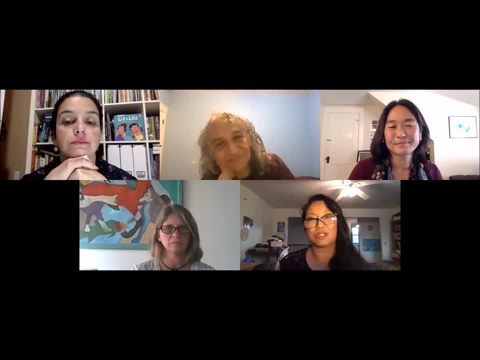 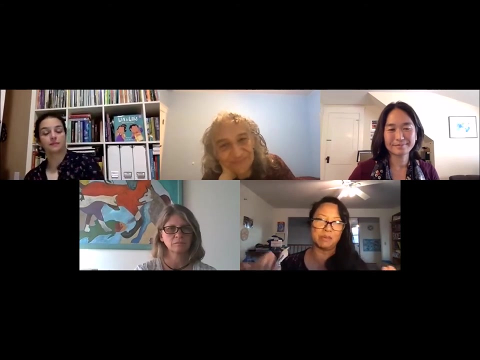 less well known um, but introduce them to some new food? or should we use a dim sum item that is more familiar to the American um population? and so I think we settled on pork buns, because it was you know um many kids have heard of a pork bun, so we thought that would be a good item to 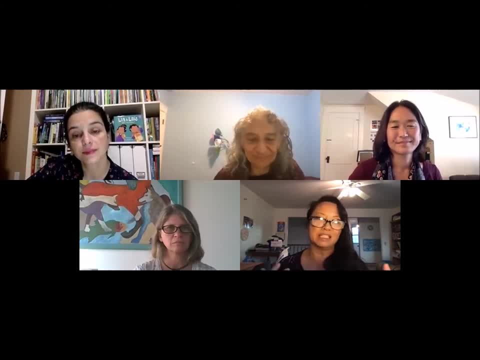 to share. uh, and then we, we kind of then, Marlene and I had a discussion about: well, is it easier, is it better to share? have five kids share figure out how to share three pork buns, or do we have three kids learn how to share five pork buns? 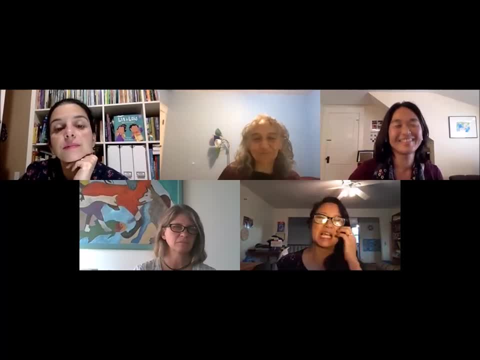 and you know which way should the math go, and so I think those are really interesting discussions. um, and it was, you know, definitely an eye-opener for me in terms of the math and trying to weave the math in. um, so can I, can I share my screen now and I? 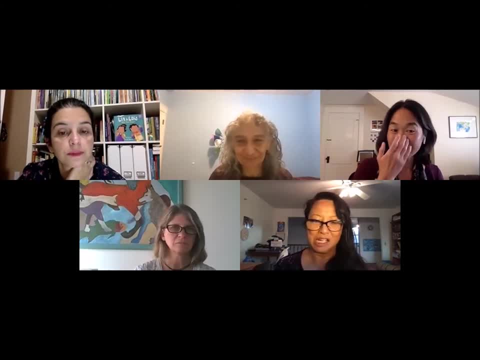 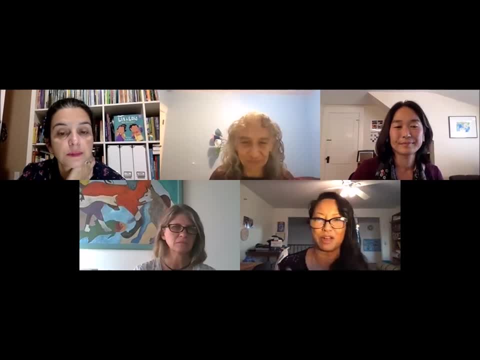 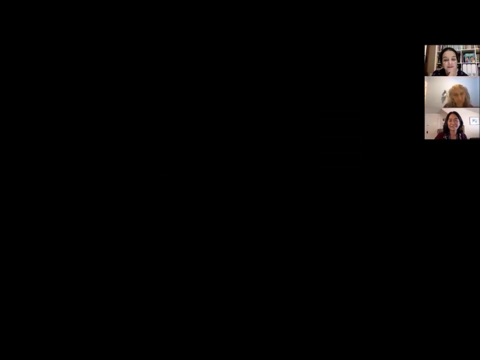 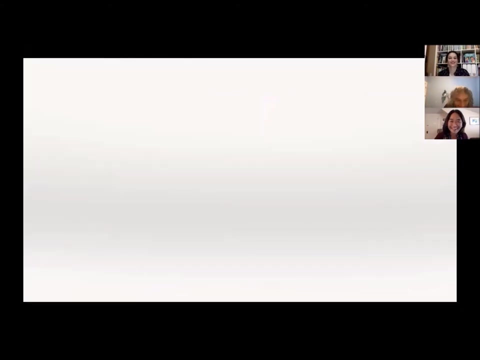 wanted to share, uh, the part where I was trying to figure out the math piece, and then I'll go into the the story and read a few pages, Okay, so I wanted to share this because, oh, I see that. 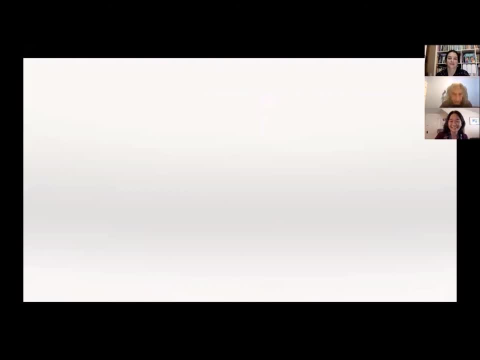 So this? so the one on the left is, uh, the illustrator, Violet Kim's. um, this is how she's figuring out, you know, the dim sum and all that kind of stuff. and we just lost it, didn't we? 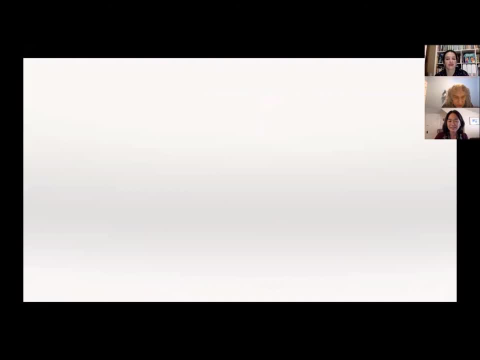 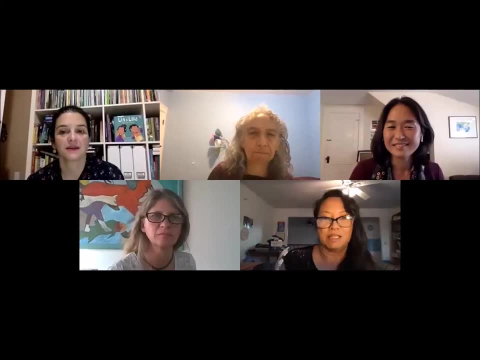 Sorry, it's Natasha, you need to go back. We saw the picture, but now it's blank. Ah, okay, wait a minute. Oh what? I don't know why this is, but I always have to share screen. Let's see. 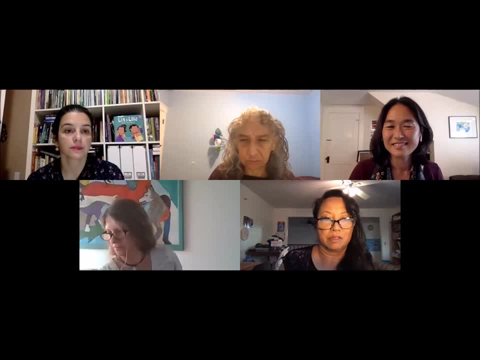 Um, okay, oops, this is it. oh, no, that's not. it wait, I completely lost the hold on a second, so sorry about this, you guys, I have don't know what happened to my PowerPoint. 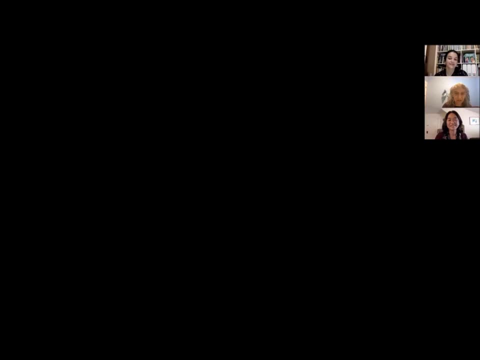 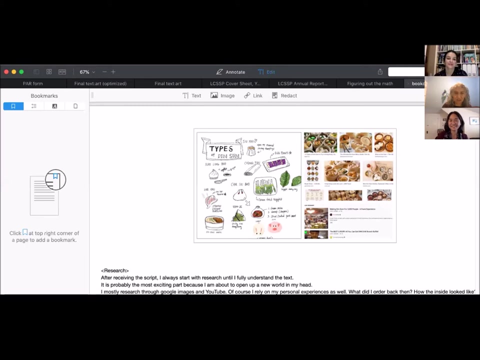 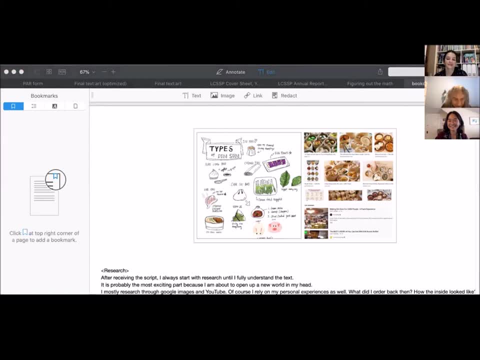 oh no, that's not it either. here it is okay. I think I have to share. um. I had this oh play, oh play slideshow in Windows. there we go. sorry, I can't find it. 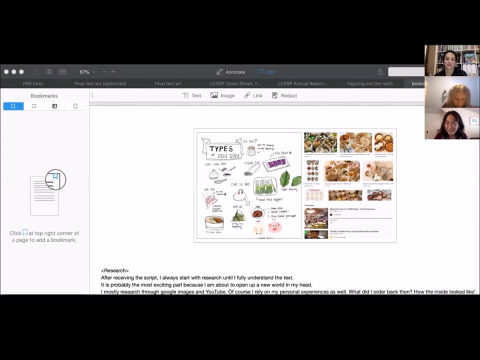 let me show you there we go. can you see? can you guys see that? now We can see the types of dim sum and the sketches and then some photos. okay, and then your notes underneath: Okay, can you guys see this now? Okay, 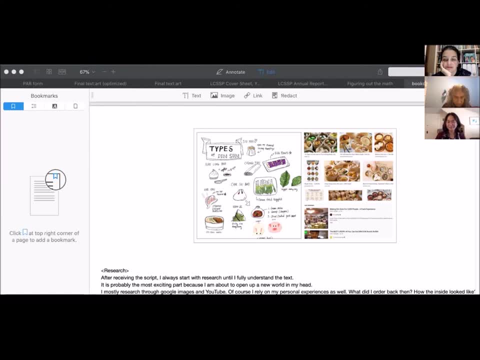 so this is my illustrators, um, working out the different types of dim sum, and then this is me, so, so I'm like trying to figure out, okay, how do we divide the pork buns, and you know. 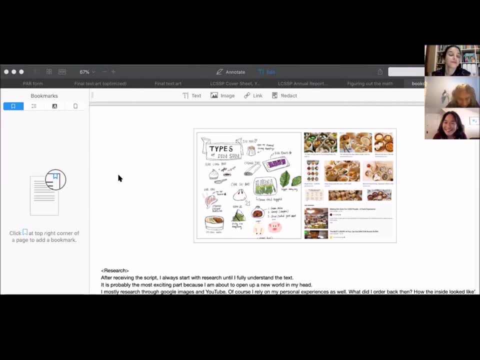 so, and I have to say that I am, uh, in addition to being math challenged, I am also artistically challenged, so that's, that's what you see. so, um, so I'll go back and just read a couple of. 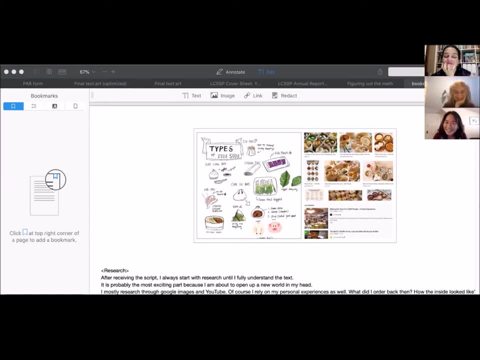 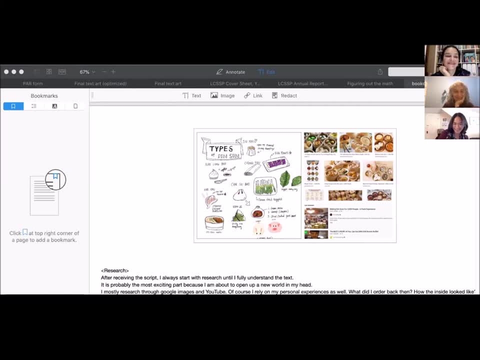 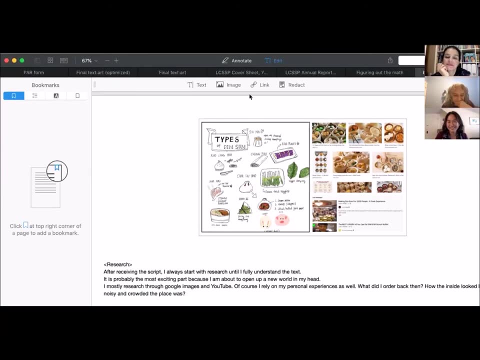 know that's, that's great. I love seeing the back story, yeah, and she just she just shared that with me, um, just the other day. so, okay, going back to let's see here. I am trying to figure out how to go back a couple pages. 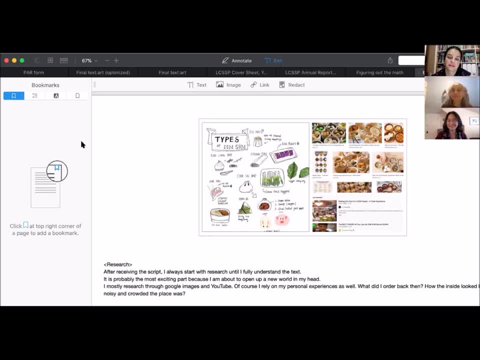 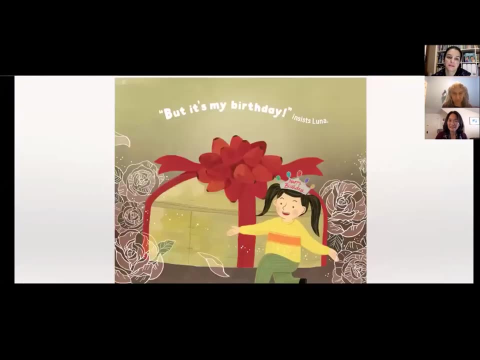 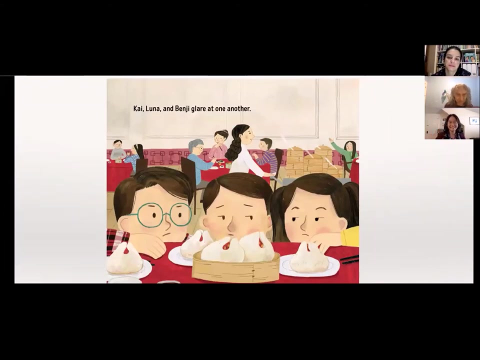 I am so sorry, guys, I did. I am kind of challenged in this department especially, um, oh, okay, there you go, okay, so. so I didn't uh. so this is the cover of the book uh, Luna's. 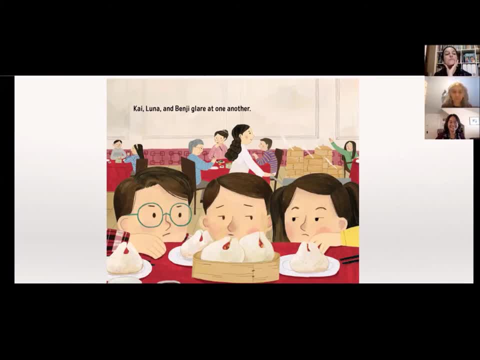 Yem, Yem, Dim Sum, and I'm just going to read a few pages. this is after they've been um, um, arguing, uh about how to share this equitably. oops, did that just okay, there we go. 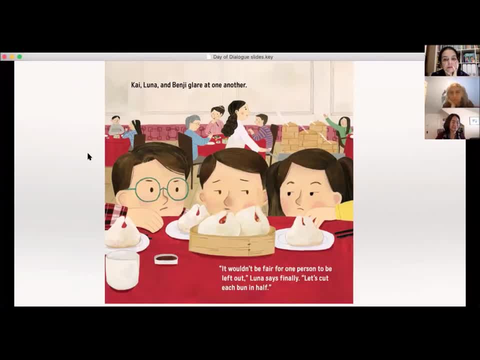 um. so Kai Luna and Benji glare at one another. it wouldn't be fair for one person, um wouldn't be fair for one person to be left out. Luna says finally, let's cut each bun in half half. 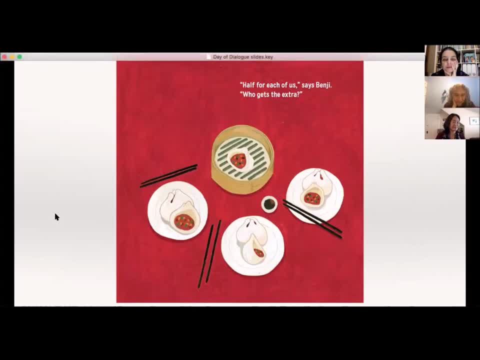 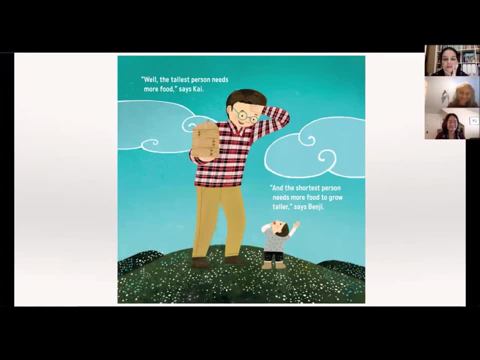 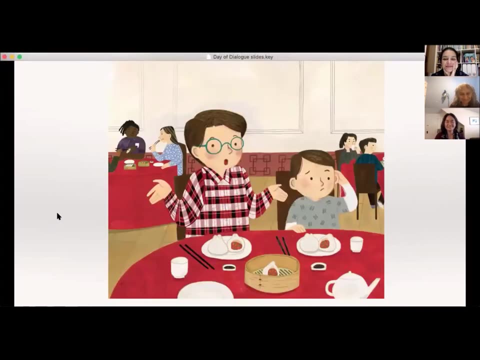 Not for each of us, says Benji. who gets the extra? Well, the tallest person needs more food, says Kai. and the shortest person needs more food to grow taller, says Benji. But it's my birthday, insists Luna. how about we cut each half in half? 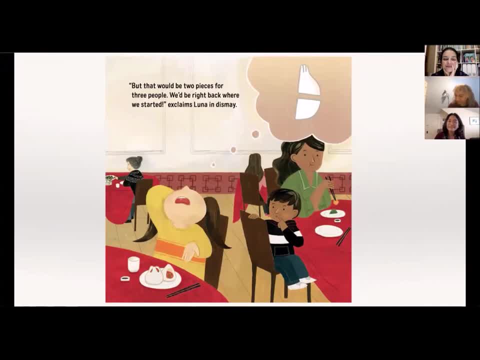 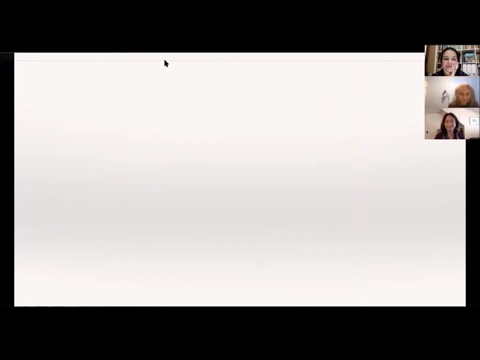 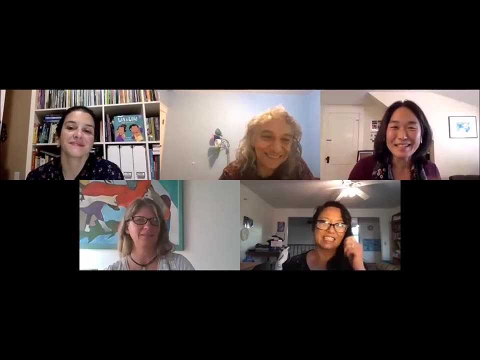 But that would be two pieces for three people. we'll be right back where we started, exclaims Luna in dismay. Oh and that was it. Thank you, So, um that. so yeah, I mean I just love the problem in the story. it's, it's so kid-centric. 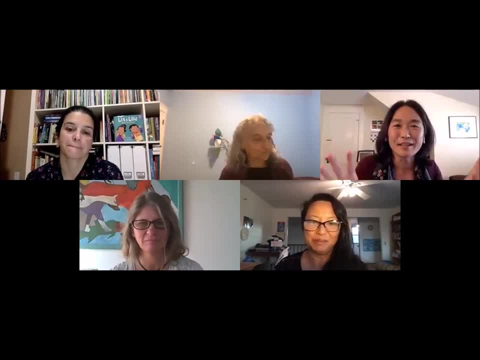 you know, they the kids. there are three kids. they have six dumplings and one falls on the floor flat, and then they have five dumplings to share between three kids, and how do they do it? Um, so, Marlene and Natasha, could you tell us a little bit about how you guys got together? 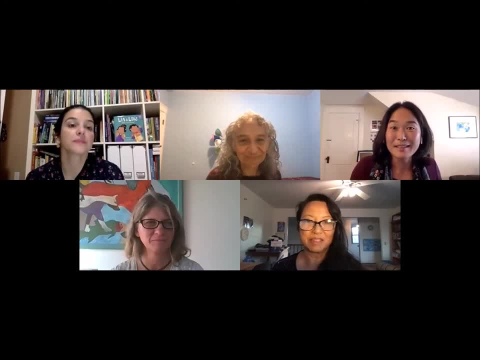 Yeah. So, Marlene and Natasha, could you tell us a little bit more about some math, that math in the story, and why it's important for kids? Well, I think what one of the things I really love about this story, and I think it's true. 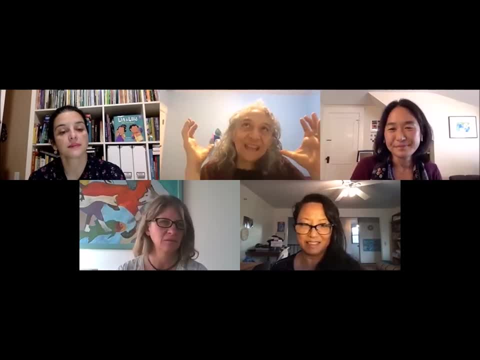 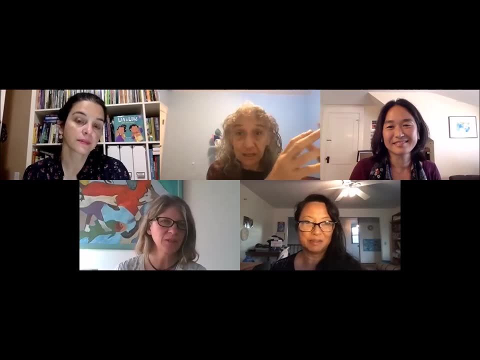 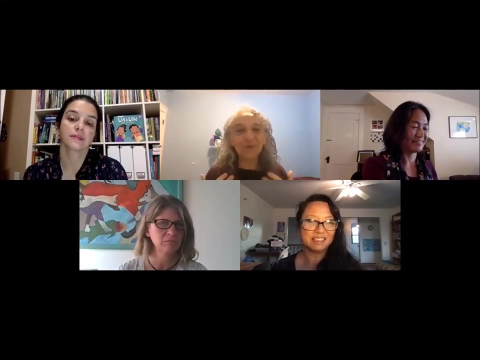 of all of our stories, but it's so accessible at different levels. so at the very start: um, there are three, sorry, there are three. three buns in a basket and two baskets. so So you see them out there. It's really obvious. Everybody knows that you know one, two, three, one, two, three. So you can get a reader who's two years old who recognizes that each kid gets one and each kid gets one. again, Everyone has two. It feels very accessible to all ages. 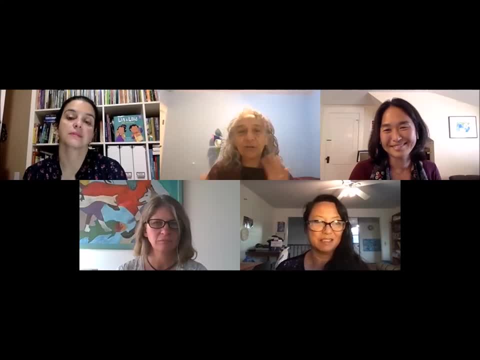 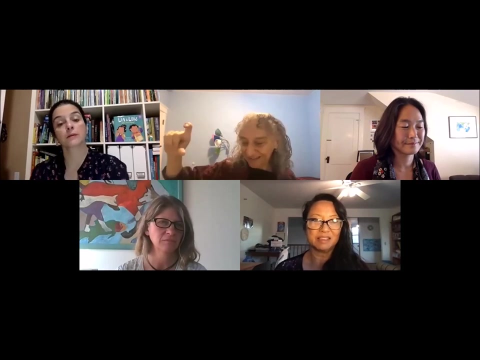 But then one falls on the floor and they go through a lot of thinking about dividing things up. What does it mean to divide something up? And that piece that you left with that page of: well, everybody gets one and a half, We have two pieces left. Then we'd be back where we said: well, that's actually pretty abstract, that dividing five into three parts. you could go on infinitely sharing out. 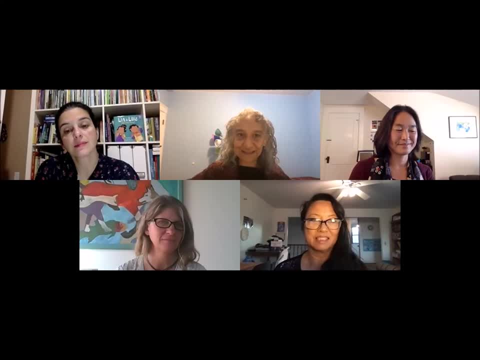 So it starts really easy and accessible and it gets pretty sort of abstract and complex. If you have a 10-year-old or a 15-year-old sitting along with a young, you know, two or three-year-old, there's something mathematical in it for all of them, from a very accessible counting to, you know, fractions, to a number theory problem almost. 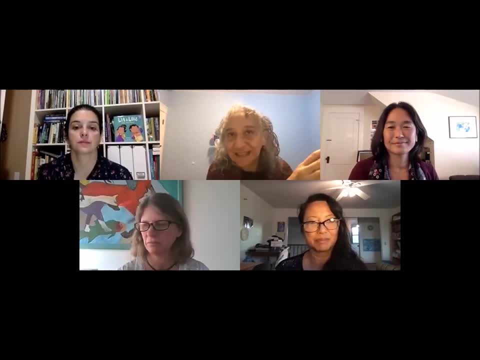 So it really gives kids this sense of what's a part of a whole, What does division mean, What's a fraction mean? They know that if you cut a half and half you get an even smaller piece. So you're hitting so much math and you're giving kids this sort of concrete reference for later years when they get to school and they meet these concepts in a more formal way. 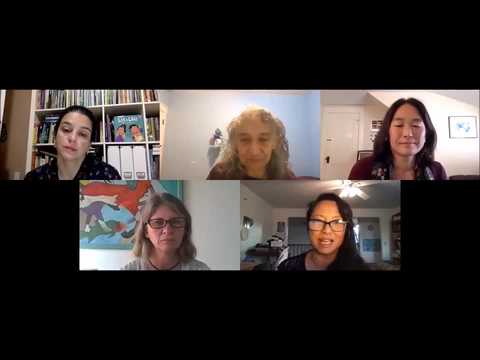 And I think the great thing about doing this with food is that kids are dealing with. you know, every day with food- I mean, you know pizza, you know it's how many kids love pizza and they eat pizza And invariably it always comes down to who gets the last piece of pizza, you know. so there's always you know the whole thing about sharing and what's equitable and how do we share this? you know last piece, And so I think there's just so many opportunities with food to figure out or have kids figure out. you know what's a part of a whole. 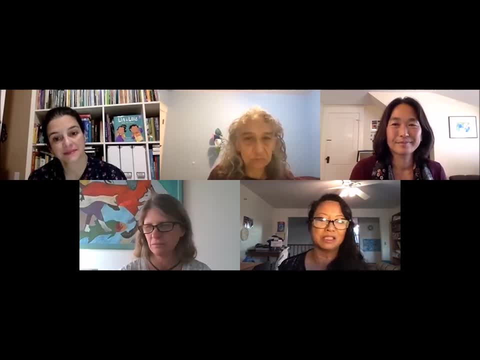 You know how do you divide things up, You know what is, and I love the question at the end of the book. I think, Marlene, that you put in there is, you know, is equal, the same as sharing fairly. you know, is that the same thing or is it different? I love that question. 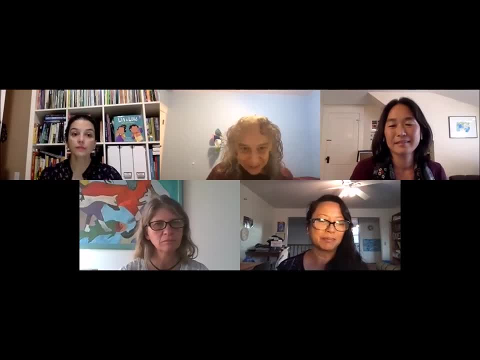 Well, that kind of also goes through the your story, where each kid is making a case for why they shouldn't be left out, and balancing that with, you know, the empathy of. well, you know, can we do this in a fair way, or should one person get more? 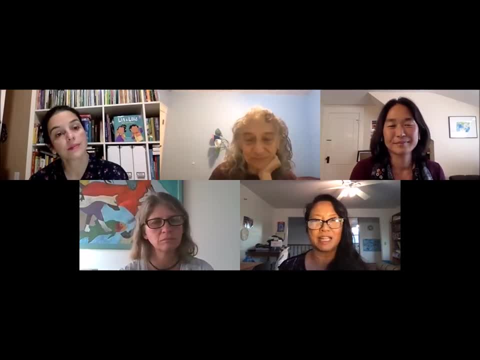 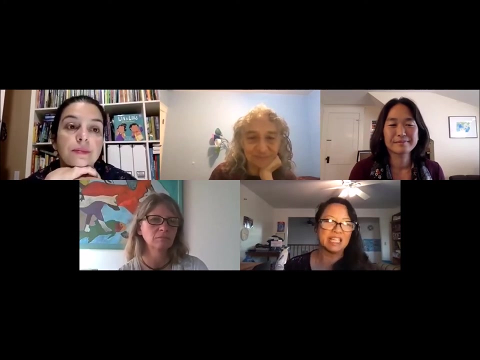 Right, And it was a great opportunity at that point to also bring in some of the Chinese culture and some of the- you know, the traditions with the lunar calendar and the animals and their place in the lunar cycle, And so that was a great place to be able to introduce that as well. 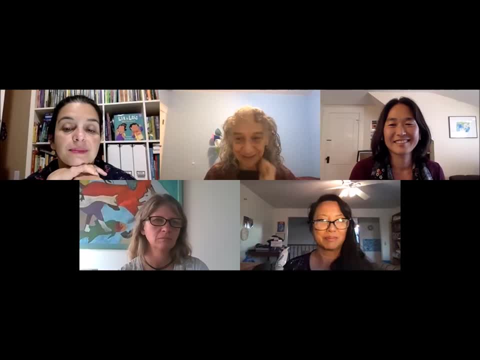 Yeah, I learned so much working with you on this book, about the animals, about what, when we were figuring out the well, when you were figuring out the foods and we were talking, I didn't know that some foods only come in baskets of this amount or that you wouldn't tend to have this this size basket. So it was very interesting to me. 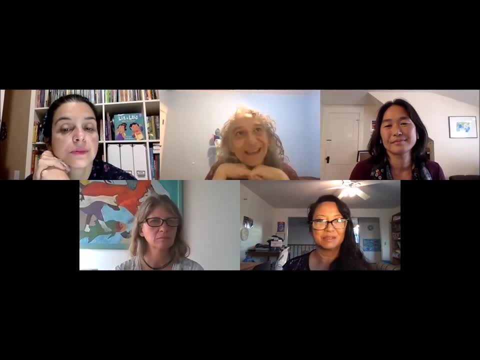 And I think it's a great argument for why We need our own voices stories, because it contains so much cultural information yet. yet it's not, you know, introduction to a holiday. It's balanced with with sibling rivalry that anybody can relate to. 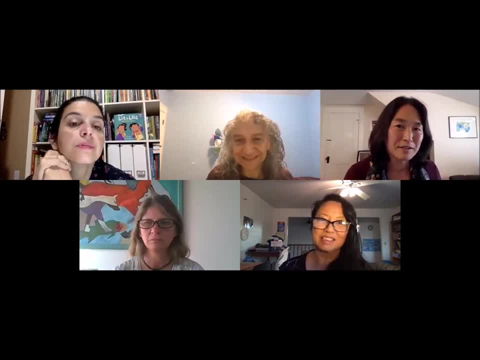 The story is going to be wonderful for Chinese New Year because there are some of those lunar calendar elements in it and they're going out for dim sum, which you could do on Chinese New Year, but it's not set on Chinese New Year. 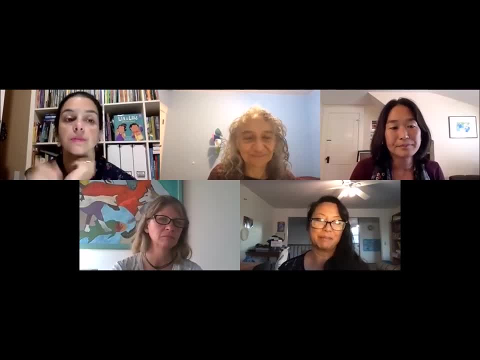 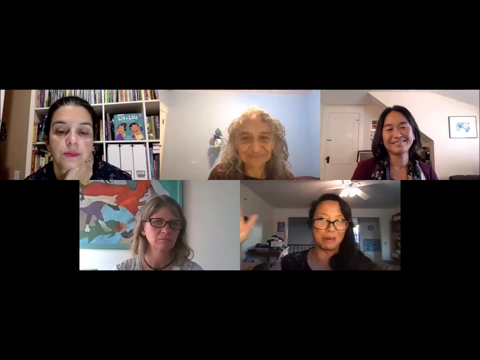 You could be reading this book any time of the year. Right, And I, I did ask my mom and my aunt, because a lot, of, a lot of dim sum dishes do come in threes, And I thought that was like some, you know, auspicious number, Chinese number thing. 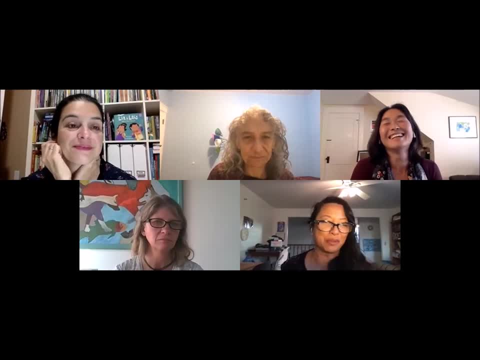 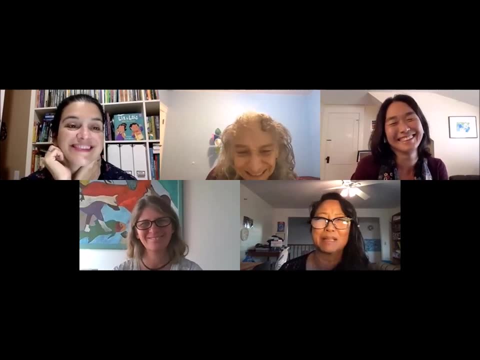 And it isn't, and nobody knows why they come in three. My mom, my mom thought you know, well, I think maybe that's just how many they can fit in a basket. Yeah, I'm like not very, it's not very scientific, you know okay. 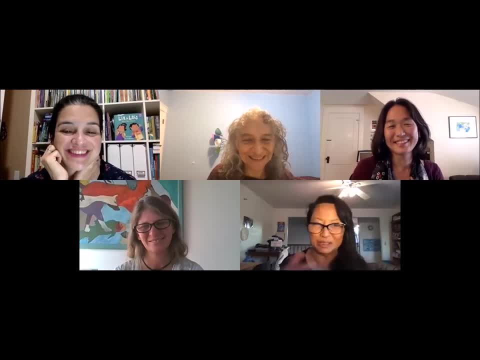 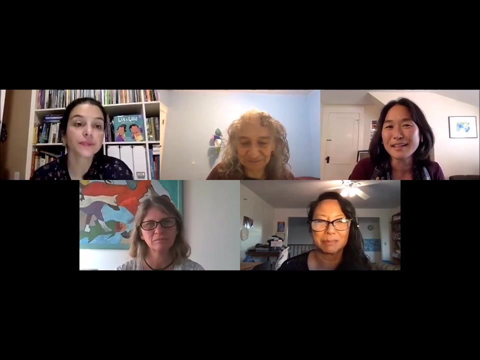 I learned some stuff too: that there is no particular reason that anyone can define why they come in threes. but Oh, thank you, Um, and any activities I can do with my. what's one activity I could do with my kids to explore the math. 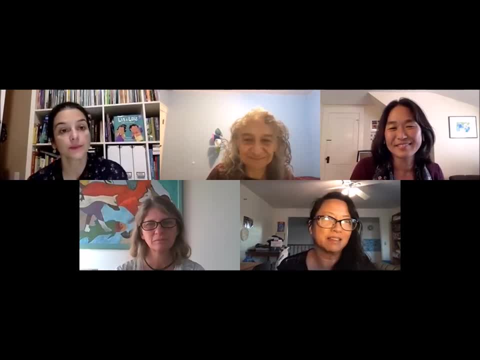 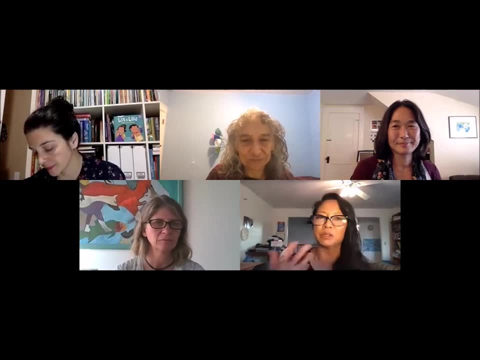 Um, I, I, I think it was you know the um, what I had um touched upon in terms of just uh with whenever you are sharing food, you know, or uh, having a family meal. 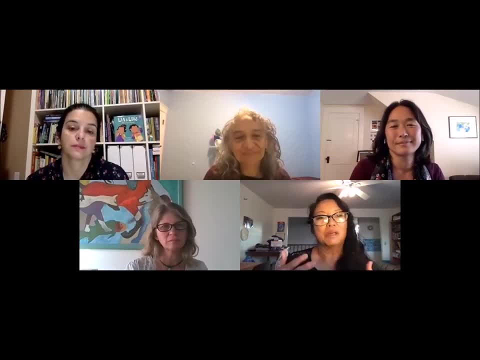 there's just like so many different ways you can kind of work the math into that, you know, and and divide things up and um, um, you know, and you can do it with almost anything. you know Play-Doh. 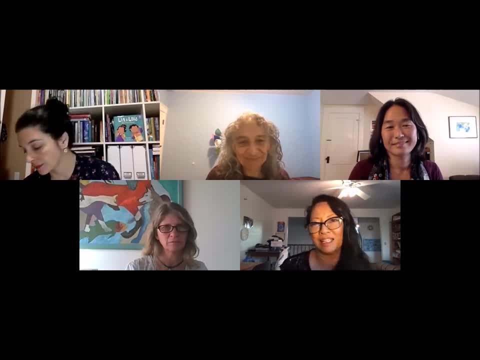 you know um, yeah, So I I think you know just sort of um asking kids questions and um you know how would you guys share this? you know apple. you know how many slices do each of you get? 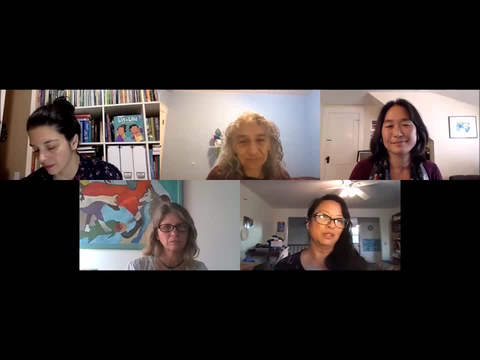 you know that kind of stuff, What did you give one piece to your brother? What? you know how many pieces are left, I mean? so there's so many different ways of incorporating that into just your normal daily um activities, and especially around snacks and mealtimes. 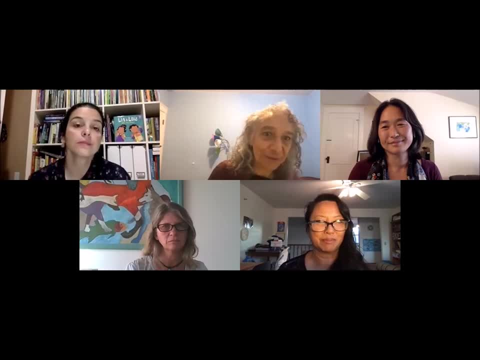 I, I agree, And I think the real life stuff of: well, maybe somebody's not that hungry, or maybe somebody's not going to eat that much because they're very young, That's all. that's all math. Again, life is not a word problem. I see in the chat here. 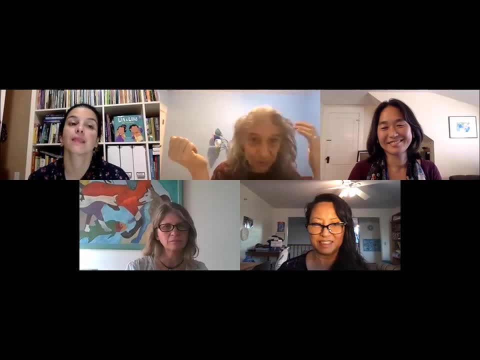 because in a word problem, everybody's getting exactly the same usually, And they're you know. but but in real life you're trying to figure out. well you know, do we want leftovers? How much is there? How do we divide it up? And imagine Dove. 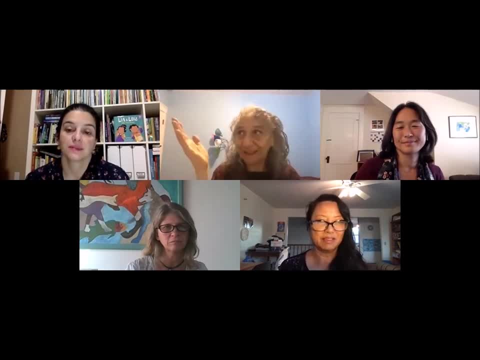 how do we divide up that pizza piece? Is they are? they don't come in nice neat, neat shape, So it it becomes pretty complicated, but that's what we deal with when you know. a lot of times I mean, I think back when my children were young. sometimes it's tempting just to say 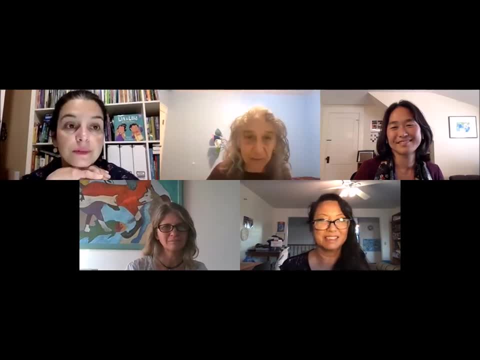 here's what everybody gets and you don't want to deal with the squabbling. but if you can turn it back on them and have them figure something out that feels equitable, um, you know, if I I give you one of my whatevers and, um, you know, if I give you one of my whatevers and you know. 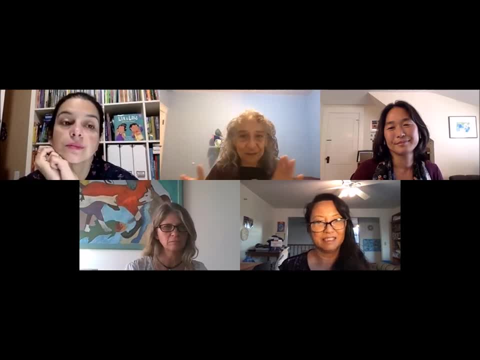 I take one of yours. it doesn't have to be a perfect math answer. Let them. let them figure out who gets what, And math will come into it somehow. I love that. Um, Erin says it's another fun way to show a math concept with a situation that is: 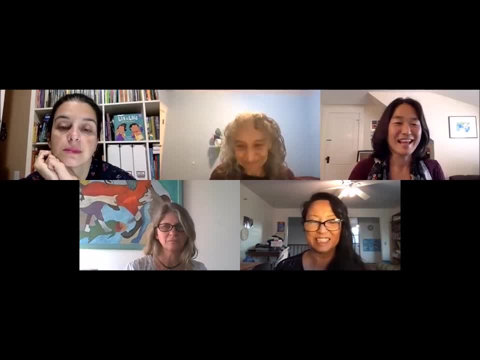 so real with young kids and siblings and parents. Now I'm hungry, Natasha Erin says And Pam Pamela says Natasha, I also live in a small town and family trips are a great excuse to eat and shop. Yeah, definitely, And sometimes unfortunately, because every time I'm with my family, 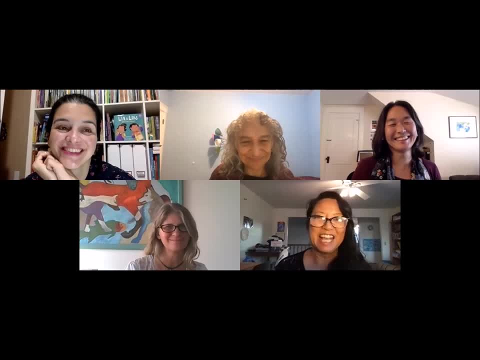 it's always: let's go to dim sum And I tend to overeat. I always tend to overeat with dim sum because I don't get it often, So You have to get it when you can. you know, Yeah, Yeah, So does. 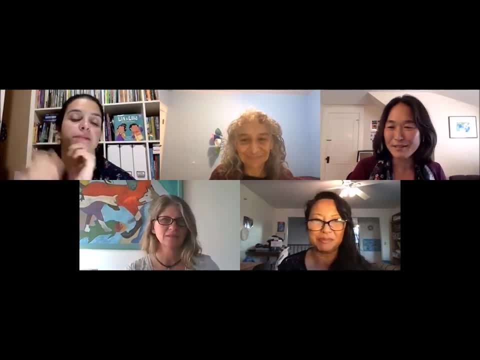 anyone have any other questions for Natasha? Um, you can just put them in the chat and I will ask them at first. Okay, So, um, it's actually 11 o'clock now. Time flew. Thank you everyone. Thank you authors. Thank you um audience. 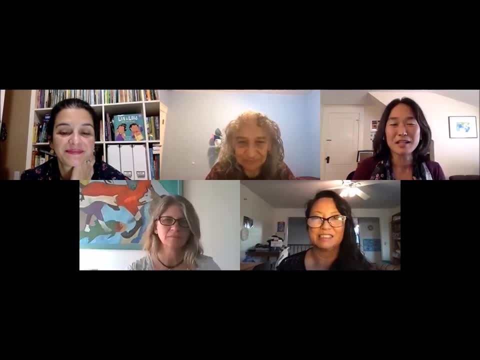 attendees for joining us. This has been such a great conversation. Uh, I know Marlene and I are going to stay on for a little bit longer, in case anyone has other questions they want to ask. Um, Anna, Natasha, Sarah, feel free to join us, Um, but otherwise, thank you everyone. It's been so much fun. Thanks. 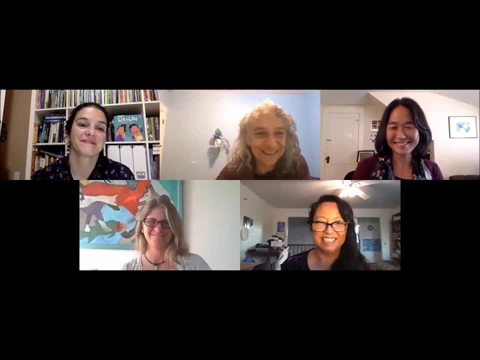 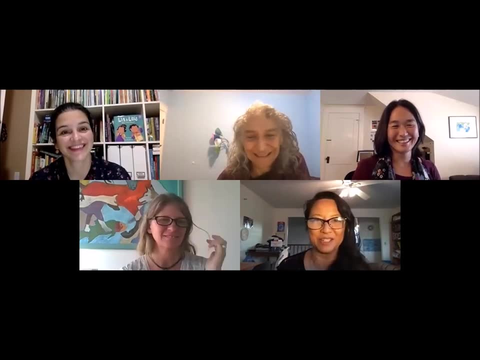 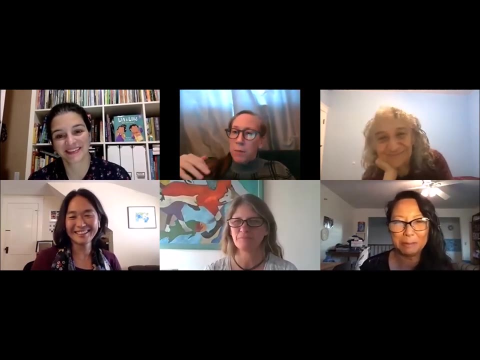 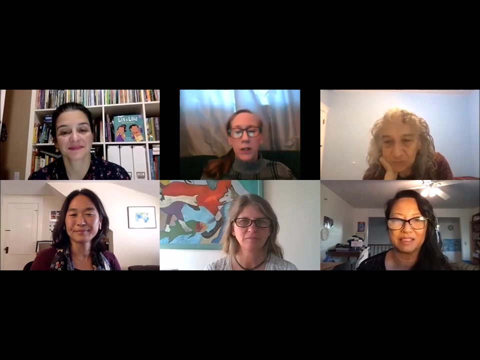 Thank you for being here, Thank you for writing all these great stories And thank you for being patient with my technology challenges. Hi everyone, Thank you, guys, so much for being here. And um, everyone. there is an activity kit for storytelling math. I put the link in the chat, but you can also get it in our booth at Day of Dialogue. um under the resources center.